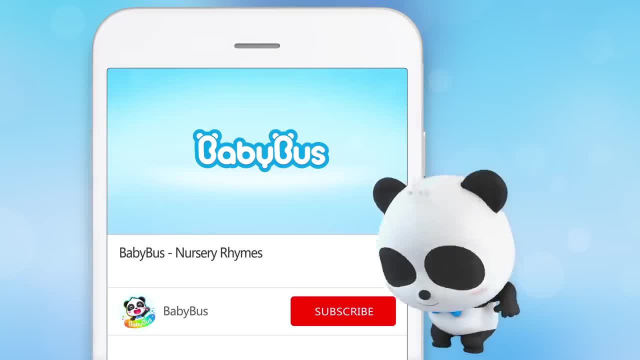 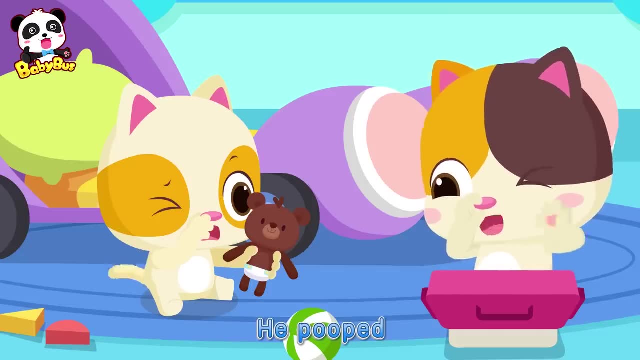 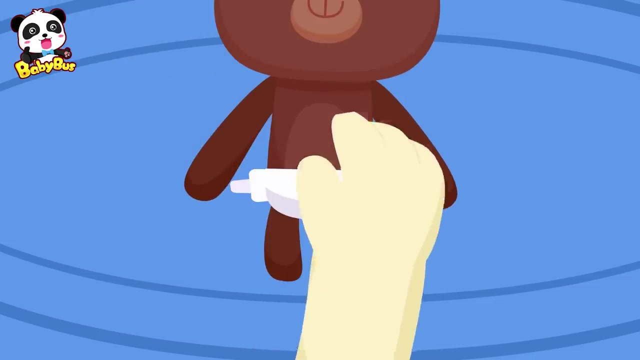 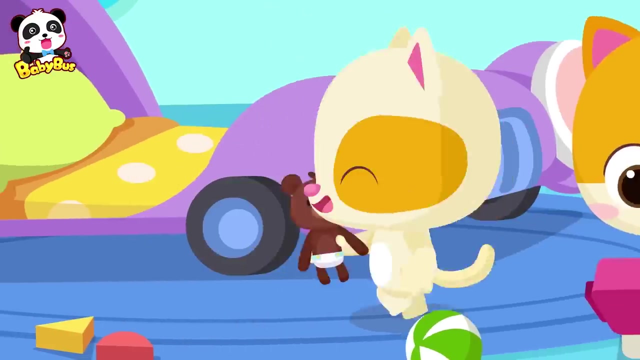 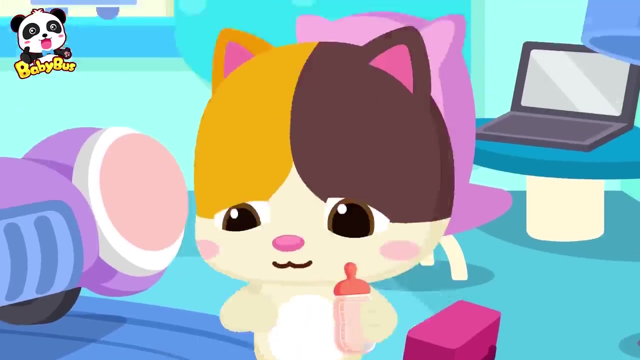 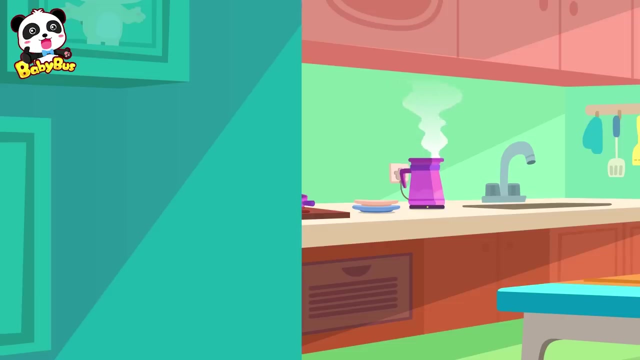 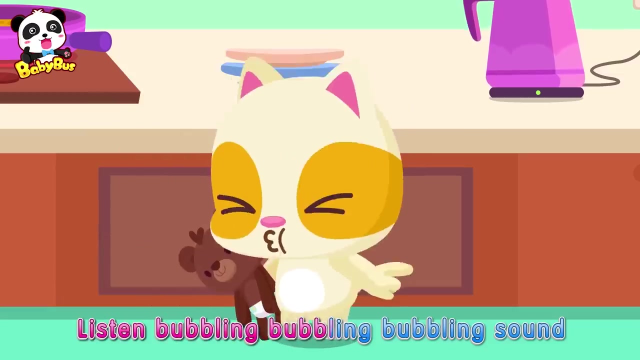 Baby Bus. Click here to subscribe. Mimi Teddy smells bad. Oh, he pooped. Let's change his diaper, Okay, Wow, Mimi Teddy is thirsty. Huh, Then let's give him some water. Okay, Listen, bubbling, bubbling, bubbling sound. 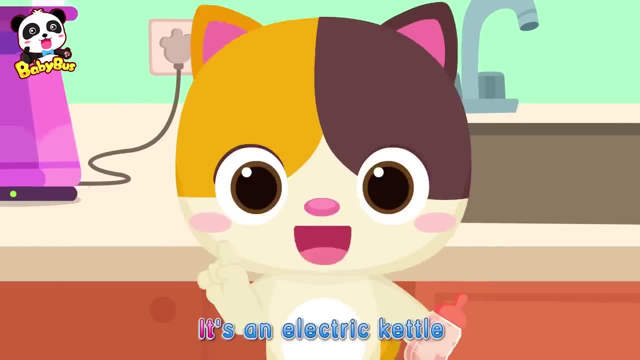 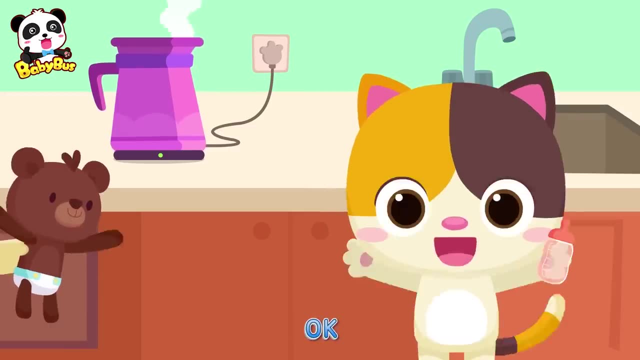 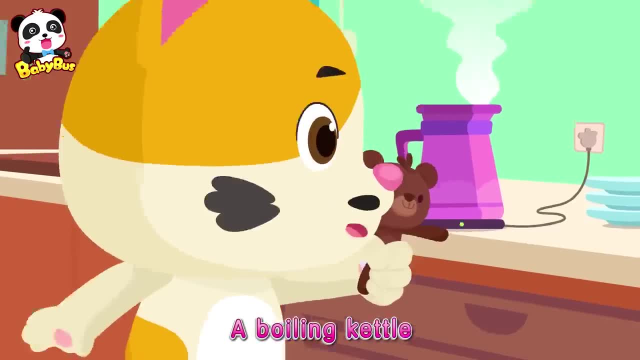 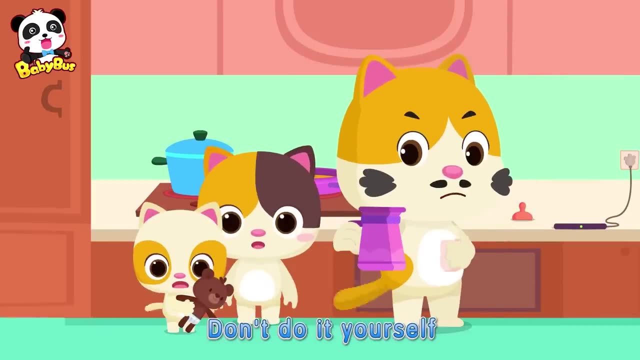 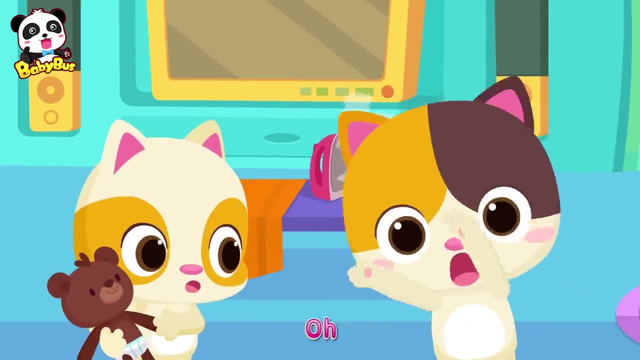 A boiling kettle. a boiling kettle. It's so hot and dangerous, don't touch it. Ask adults when pouring the hot water. Don't do it yourself. Look, spinning, spinning, spinning. oh, what is it? White steam. white steam, oh, it's an electric iron. 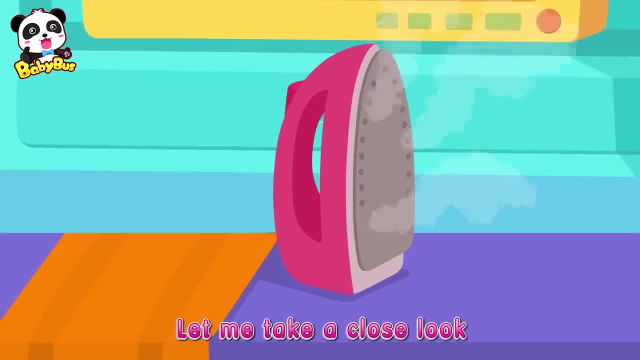 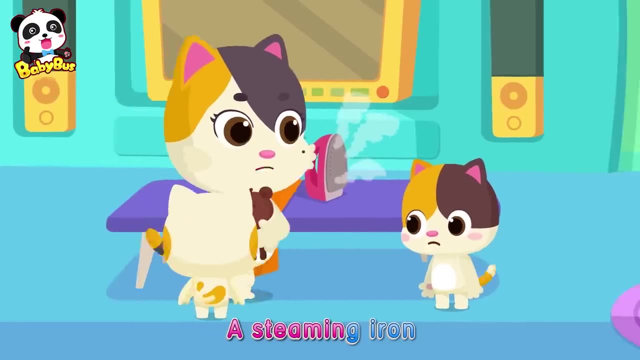 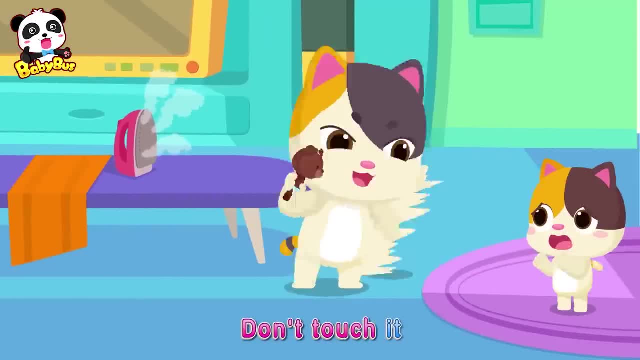 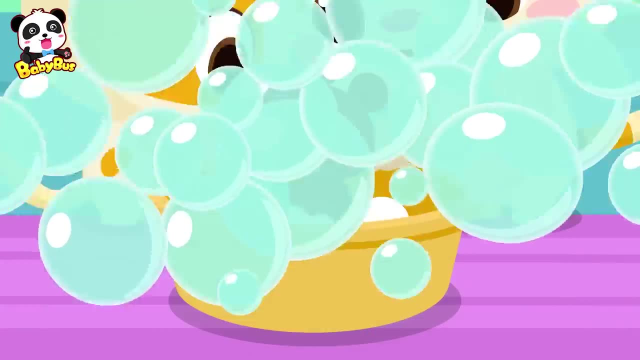 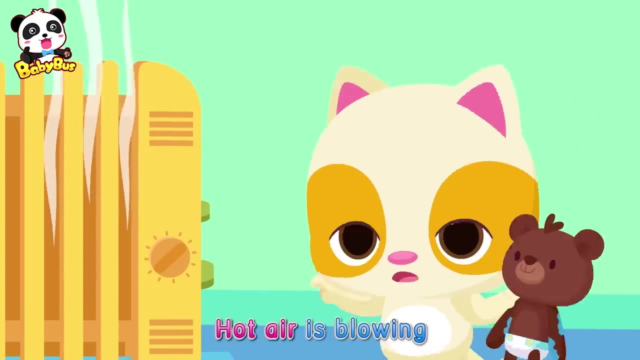 It's so hot and dangerous, don't touch it. Please stay away from hot, steaming irons. Oh, blowing, blowing, hot air is blowing. What is it? Hot air, hot air. oh, it's an electric heater. 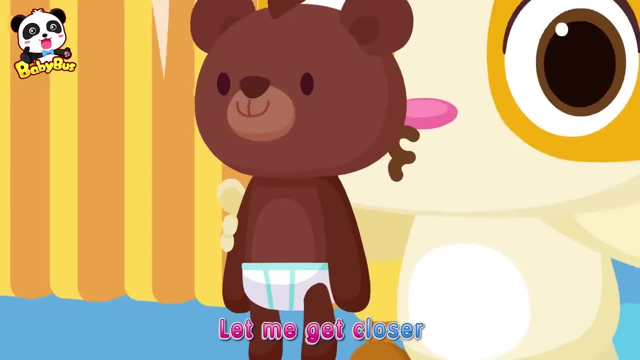 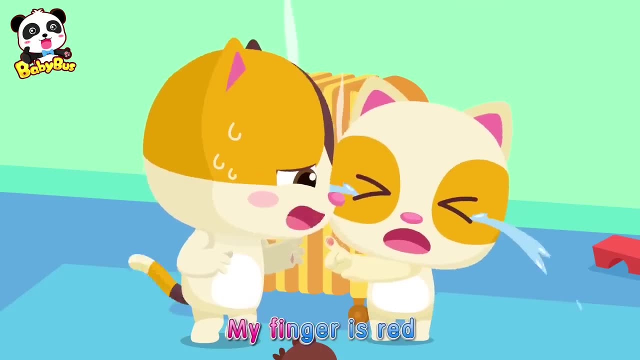 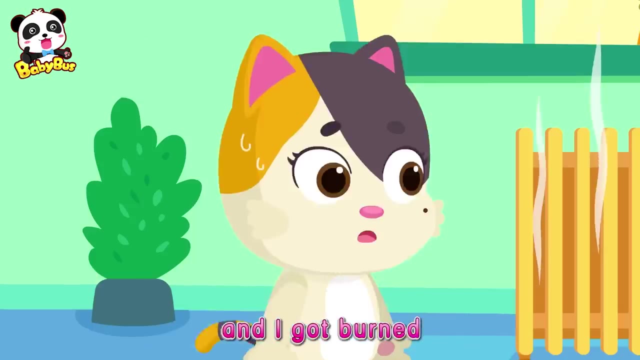 What is it? I'm so cold. let me get closer. Ouch, it's hot, Hot, hot hot. my finger hurts, My finger is red, my finger hurts. I touched the hot heater and I got burned. No, no, no, no, no, no, no, it's dangerous. 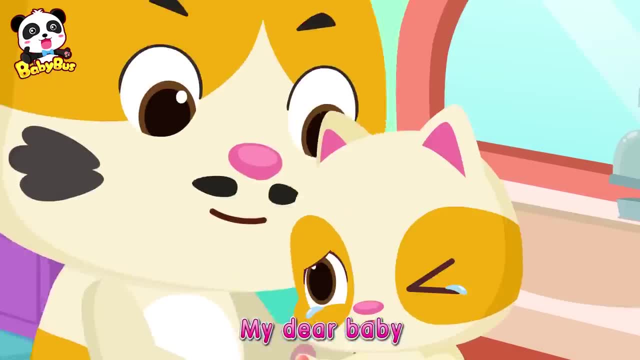 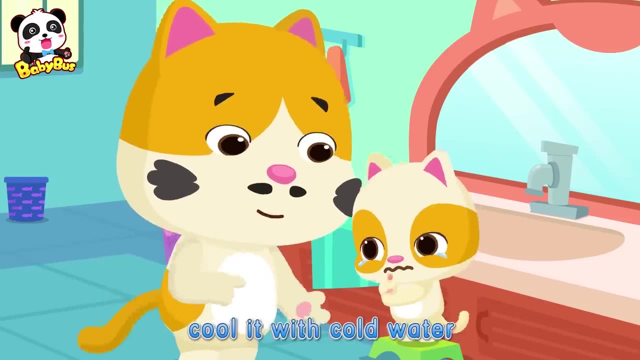 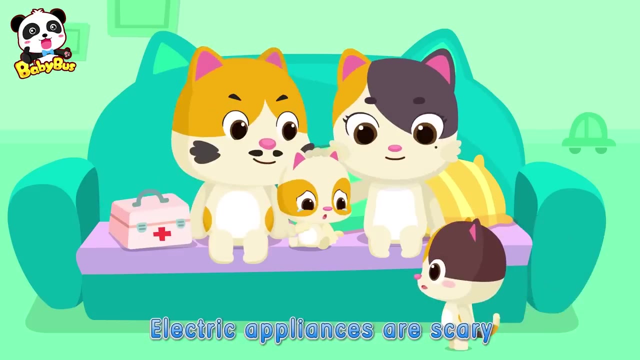 My dear baby, my dear baby, Hoo, hoo, hoo hoo, you will be all right If your finger got burned, Cool Cool it with cold water. Electric appliances are scary, So you should always be careful. 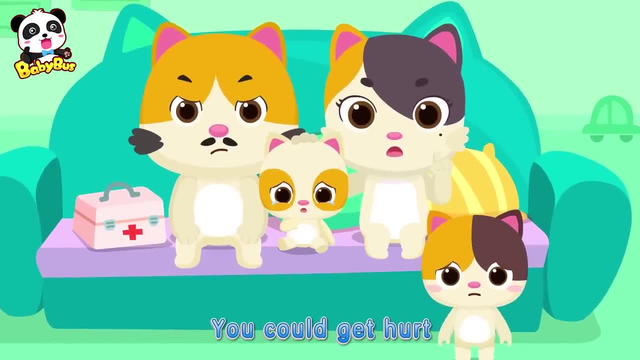 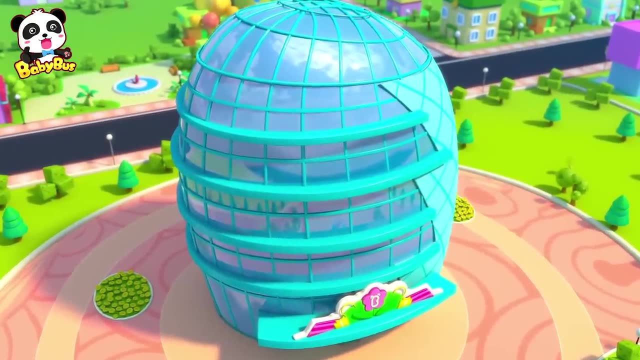 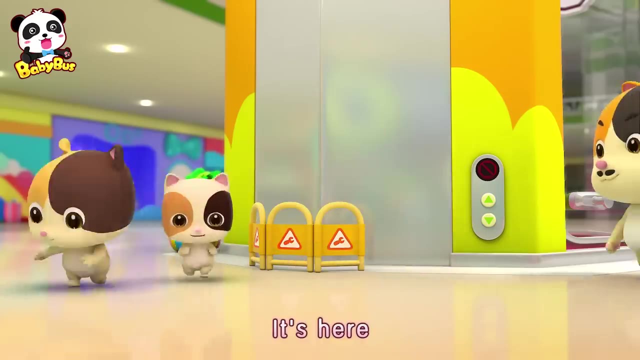 And make sure you don't touch them. You could get hurt. Okay, we got it. Elevator, elevator, It's here. It's here. What's this? Oh, it's broken. We have to go up to the sixth floor. 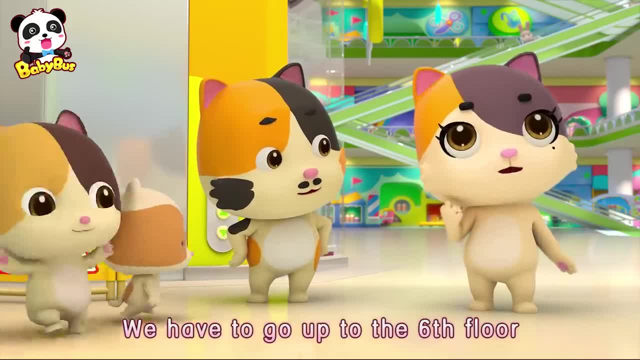 What should we do? It's so high I don't want to walk up the stairs. Don't worry, Mimi, You'll be okay. You'll be okay, I'm fine. I'm okay. I'm fine, I'm okay. 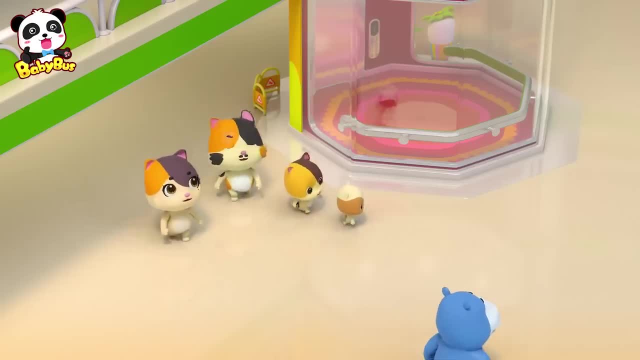 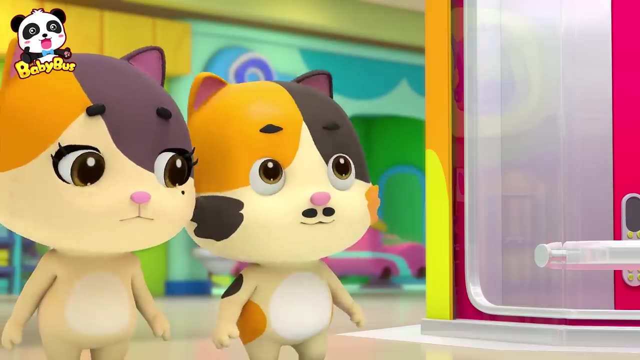 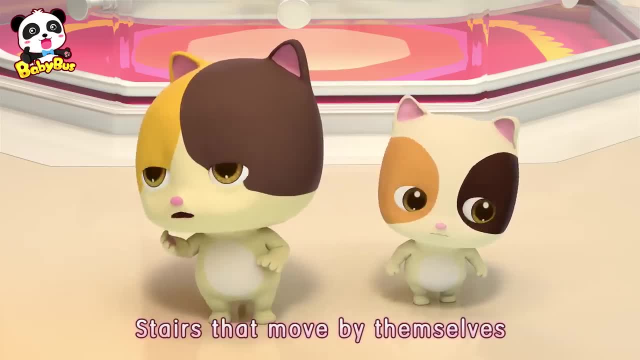 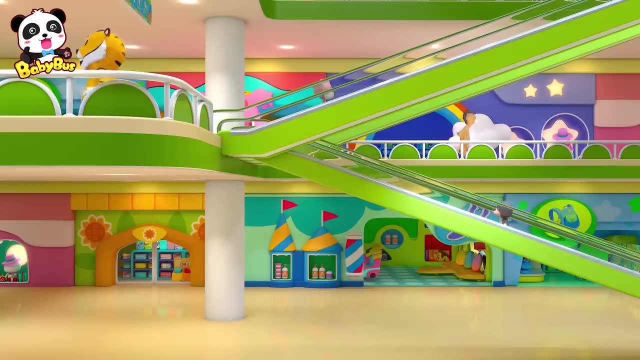 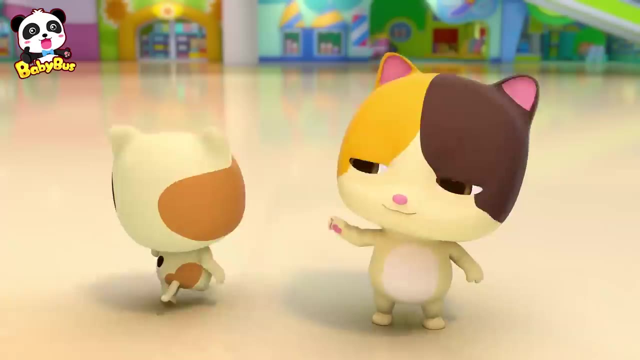 It's the好好 story, Mimi: There are stairs that move by themselves. Do you know what it is? Stairs that move by themselves? Ah, I know, It's an escalator. You are right, Escalator. 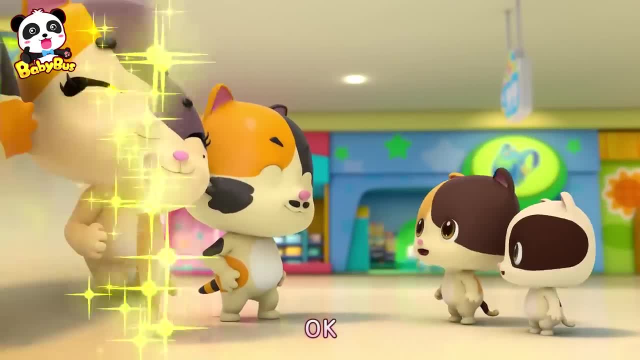 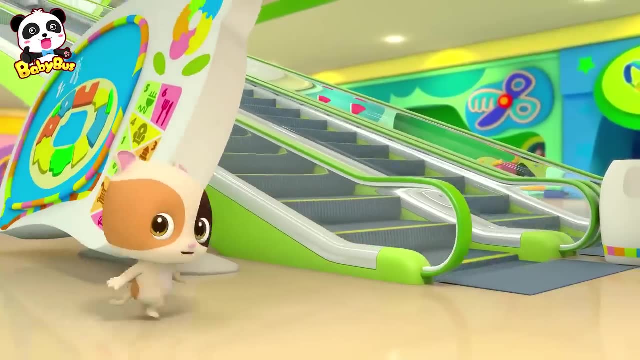 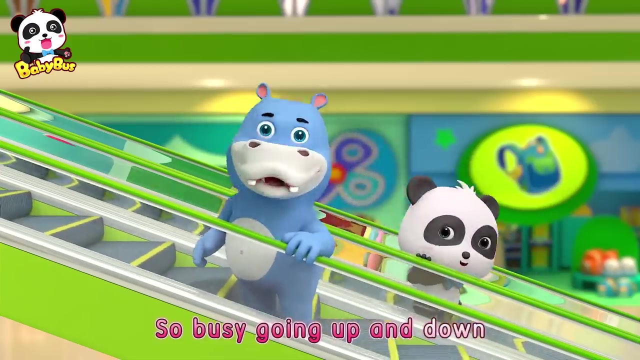 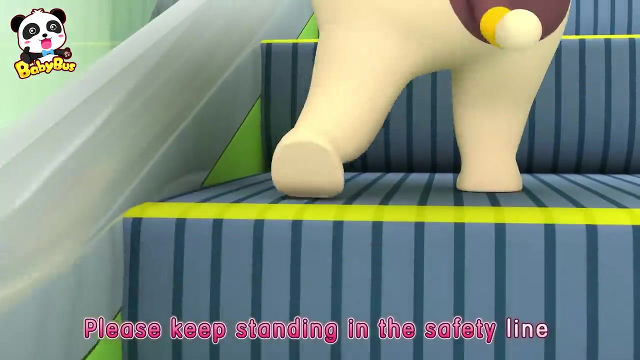 Escalator. Let's take the escalator, A long escalator in the shopping mall, So busy, going up and down. Holding mom's hand tight, and stand in a line. Please keep standing in the safety line. Please don't run. please don't jump. 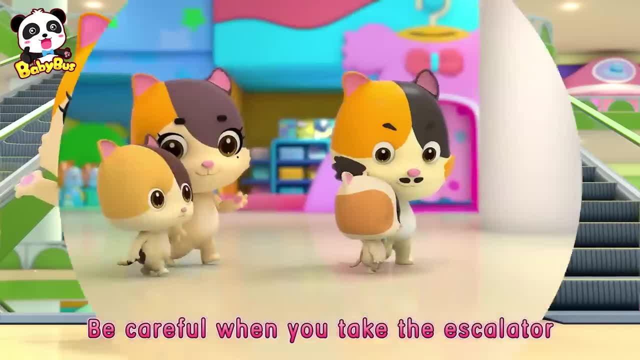 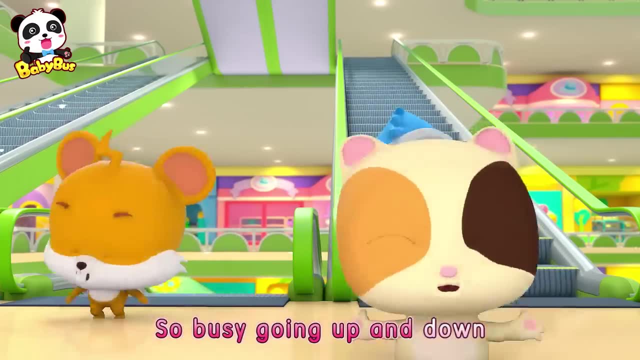 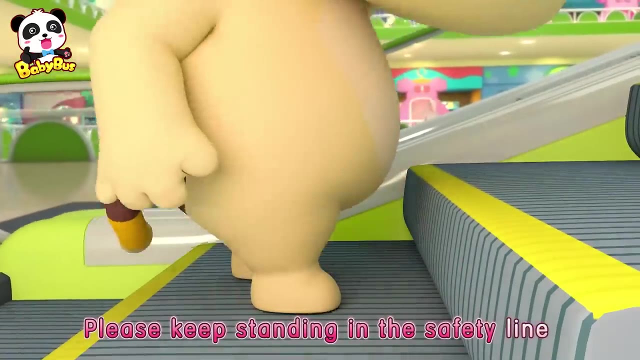 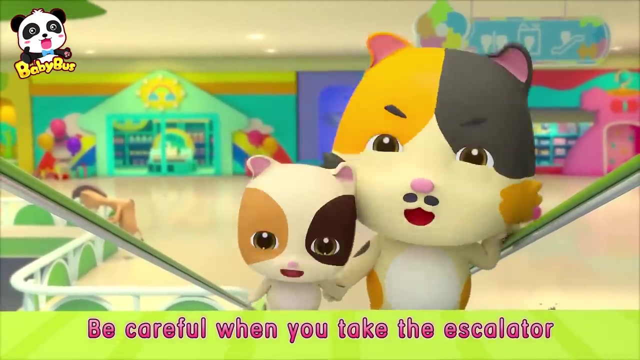 Be careful when you take the escalator- A long escalator in the shopping mall So busy, going up and down, Holding mom's hand tight and stand in a line. Please keep standing in the safety line. Please don't run, please don't jump. Be careful when you take the escalator. 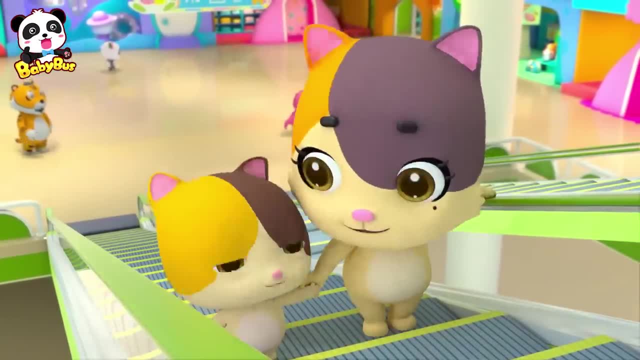 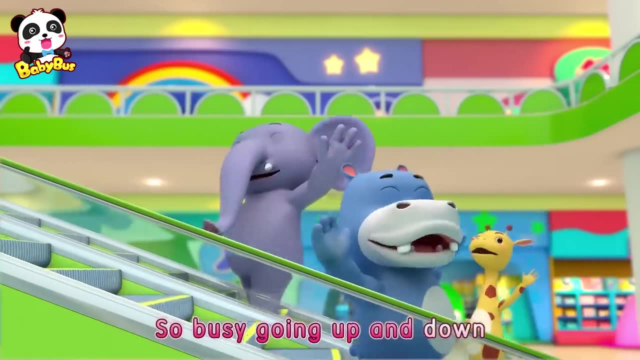 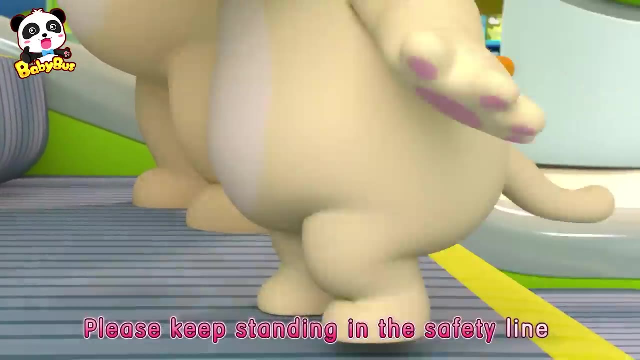 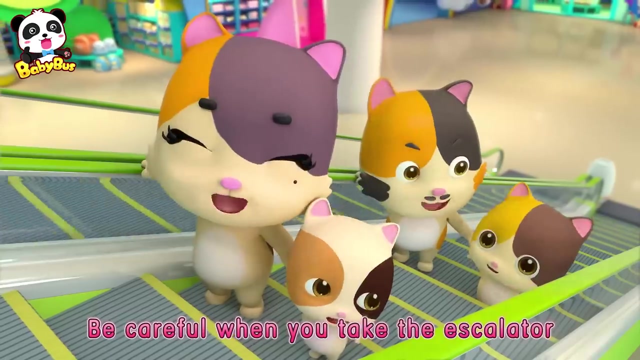 Mom, I want some toys. A long escalator in the shopping mall, So busy going up and down, Holding mom's hand tight and stand in a line. Please keep standing in the safety line. Please don't run, please don't jump. Be careful when you take the escalator. 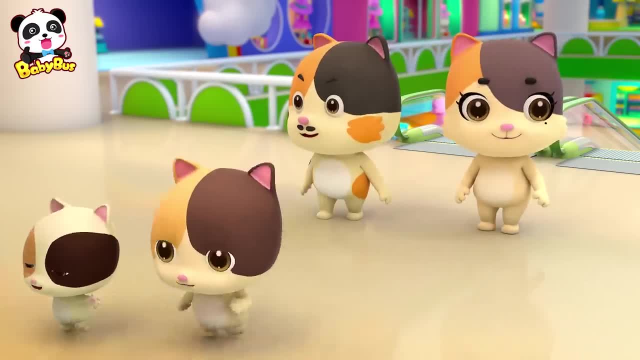 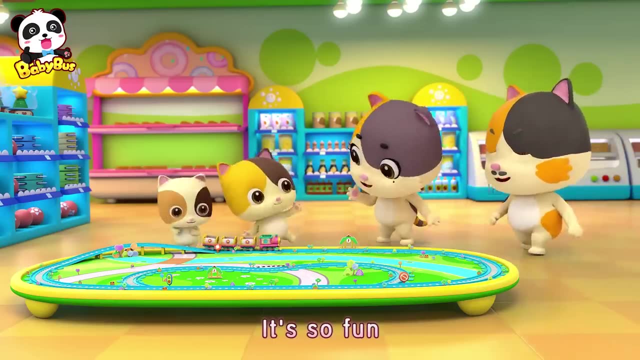 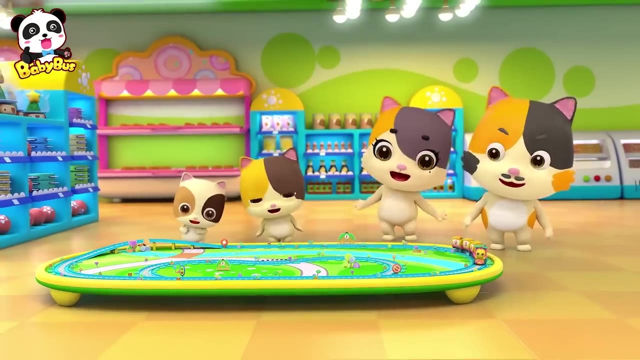 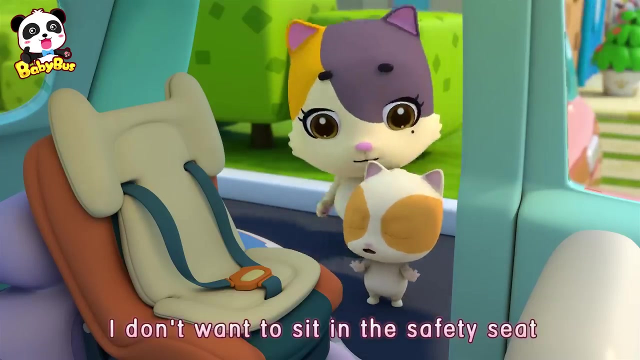 Wow, It's a toy train van. Wow, Yay, It's so fun, So fun, So fun. Yeah, Let's go. I don't want to sit in the safety seat. Sweetie, it will keep you safe. 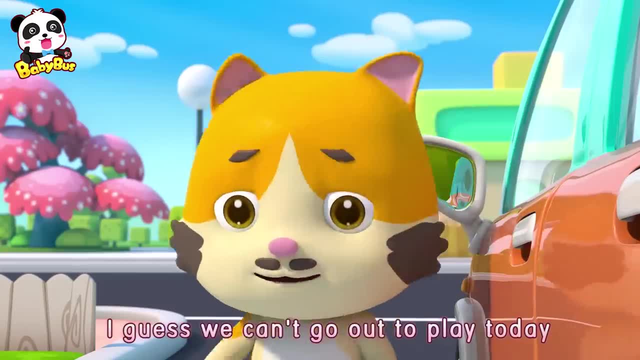 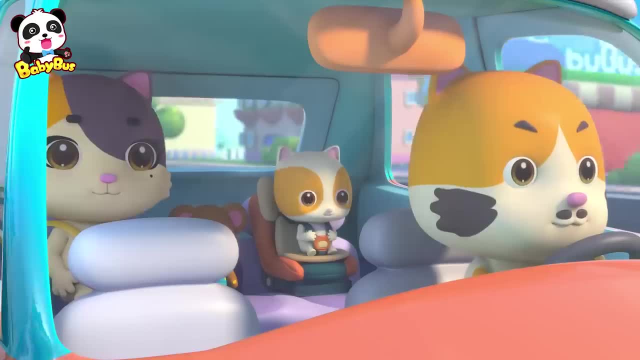 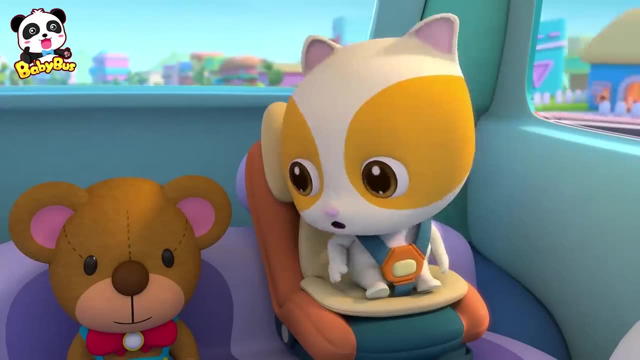 Well then, I guess we can't go out to play. Well then, I guess we can't go out to play. Well then, I guess we can't go out to play. Mom, are we there yet? Not yet, Mommy, please help me, please. 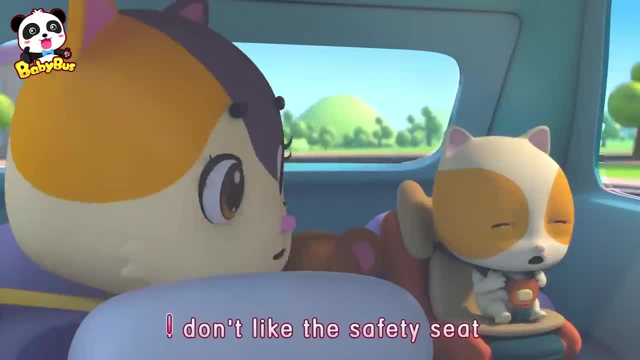 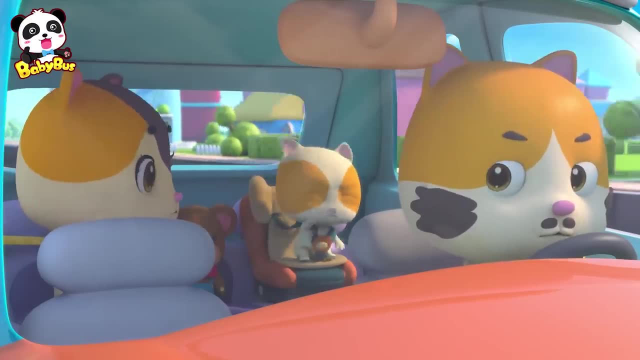 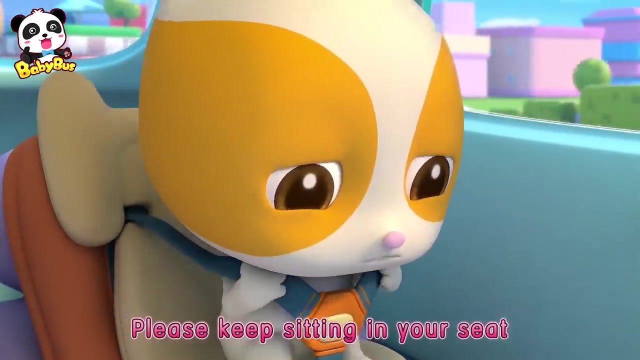 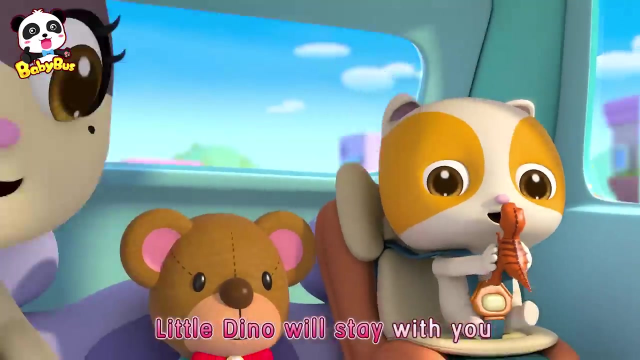 Please unbuckle my seatbelt. I don't like the safety seat, I want to get out of it. Sweetie, sweetie, sit up straight. Please keep sitting in your seat. Look what Mommy brought here for you. Wow, little dino. Little dino will stay with you. 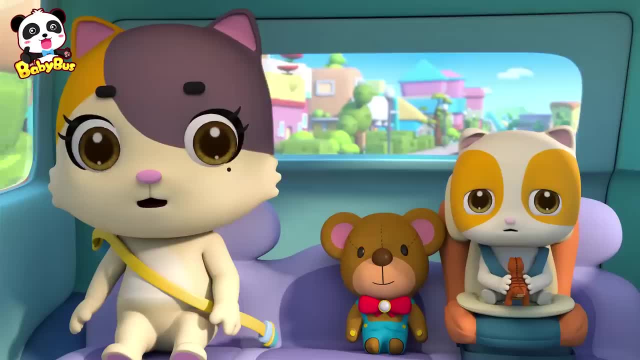 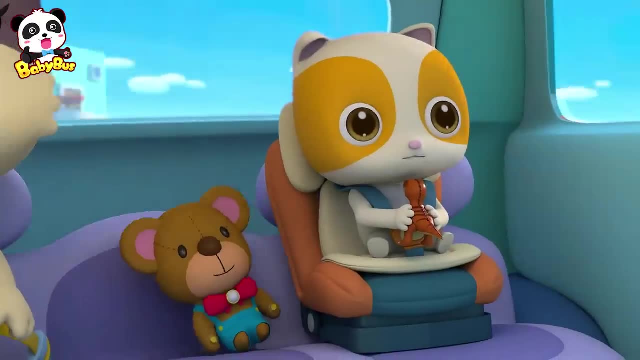 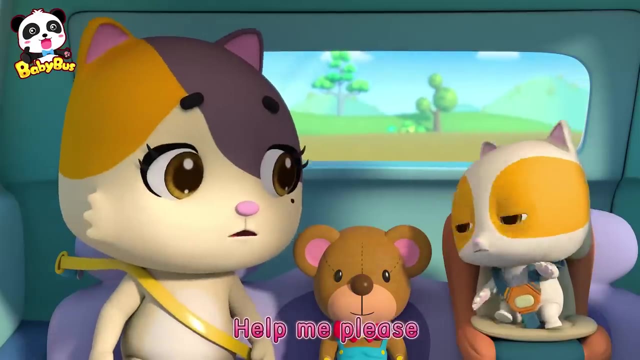 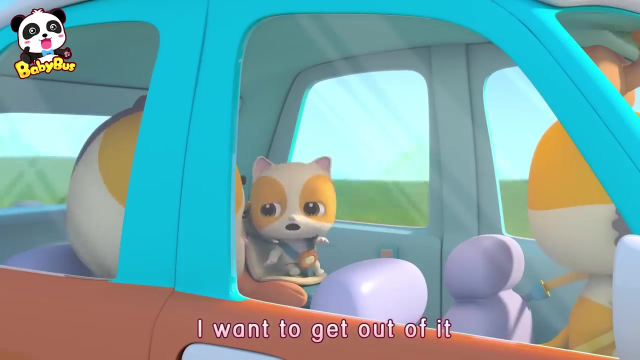 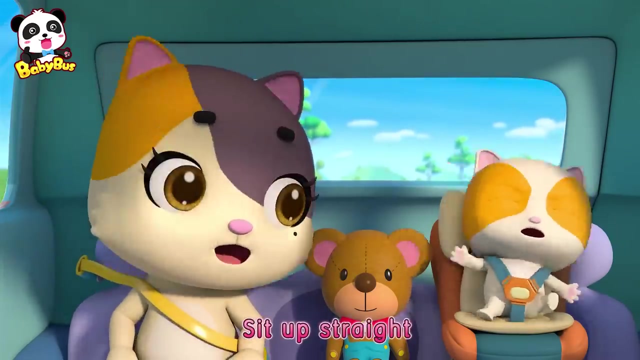 Here comes a curve. Don't worry, your seat will keep you safe. Mommy, please help me, please, Please, unbuckle my seatbelt. I don't like the safety seat, I want to get out of it. Sweetie, sweetie, sit up straight. 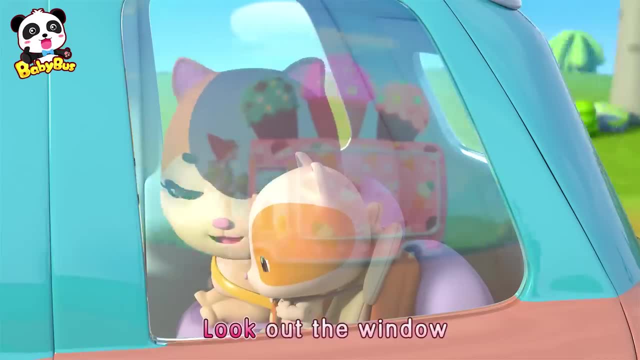 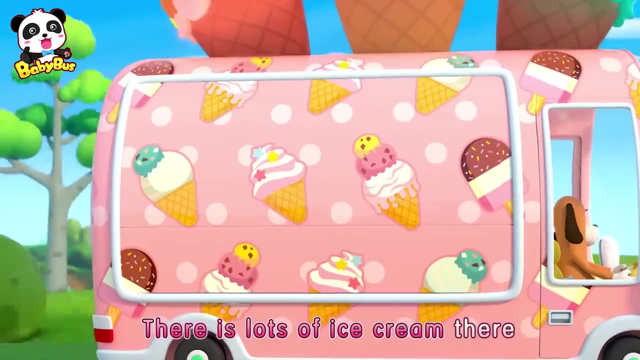 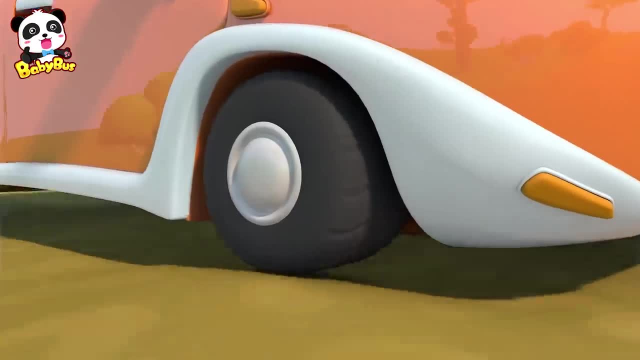 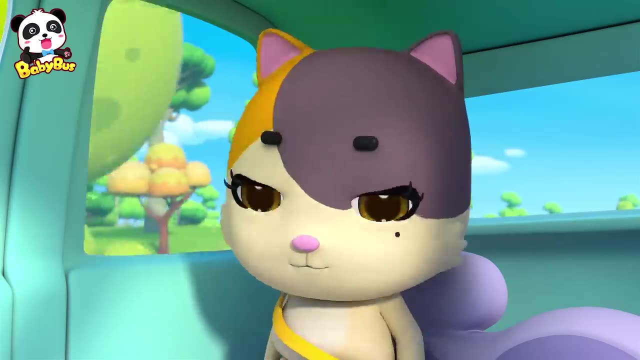 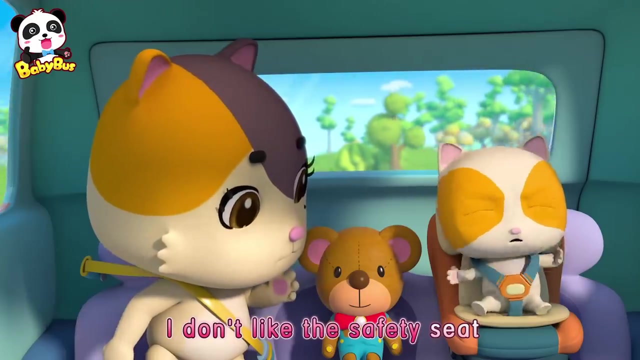 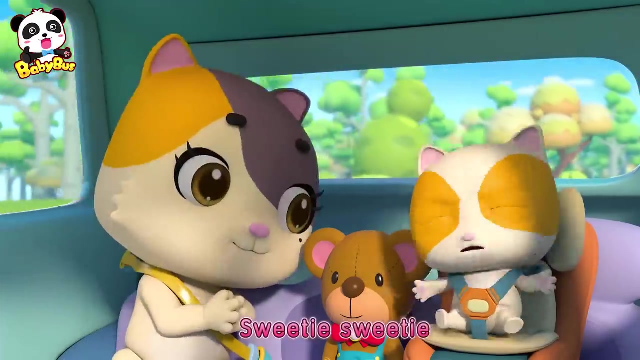 Don't worry, your seat will keep you safe. Mommy, please help me, please, Please, unbuckle my seat belt. I don't like the city seat. I want to get out of it. Sweetie, sweetie, sit up straight. 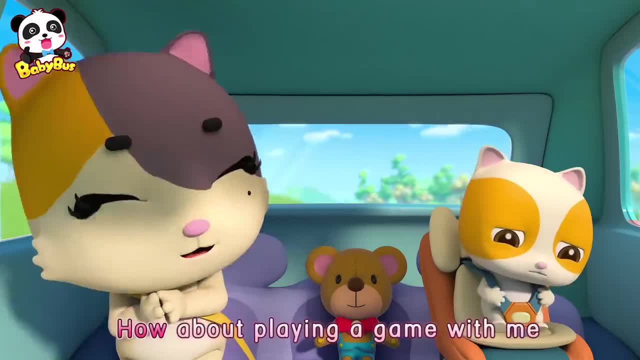 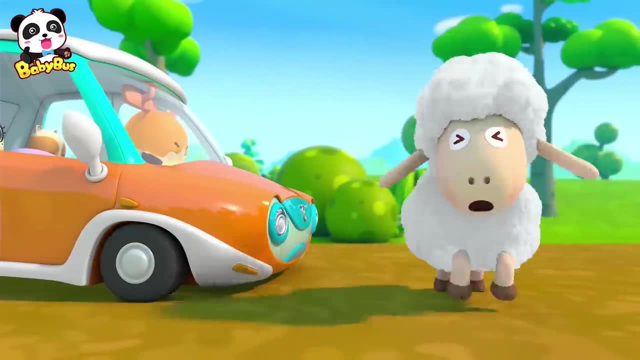 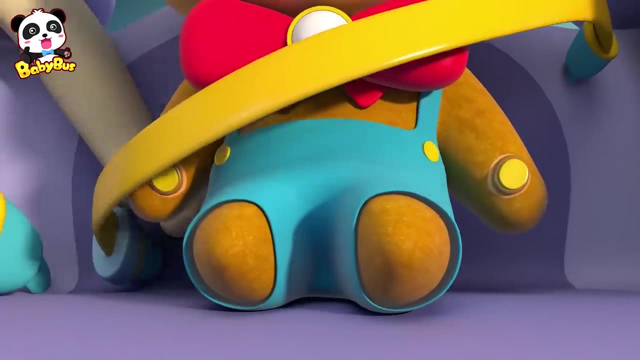 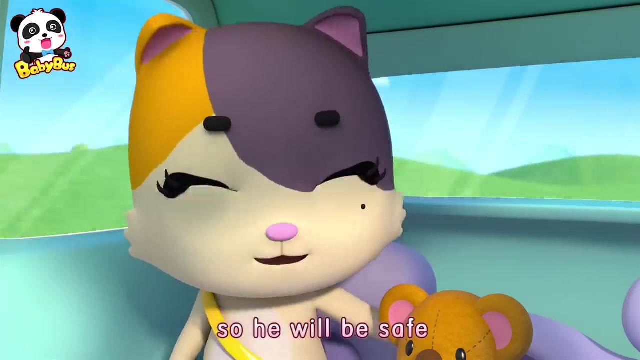 Please keep sitting in your seat. How about playing a game with me? What kind of game? Ah, watch out. Ah, my teddy. Teddy fell down because he did not sit in his safety seat. He's wearing a seat belt now, so he will be safe. 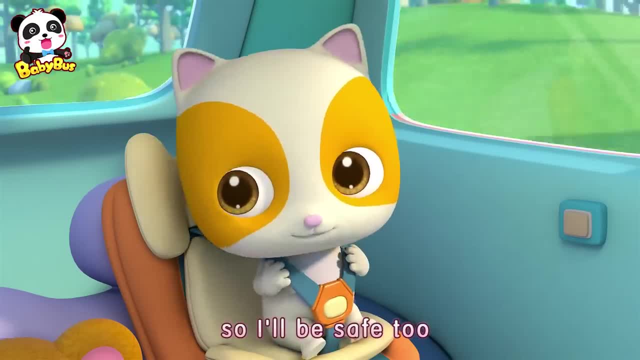 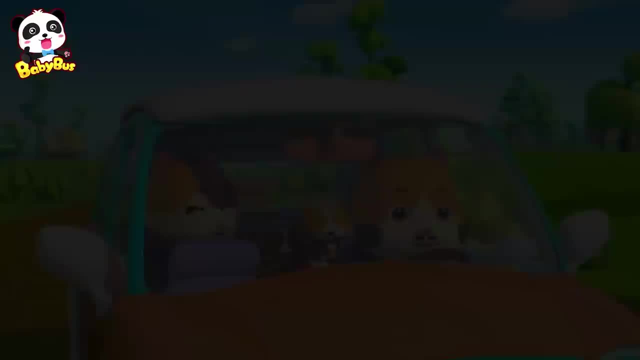 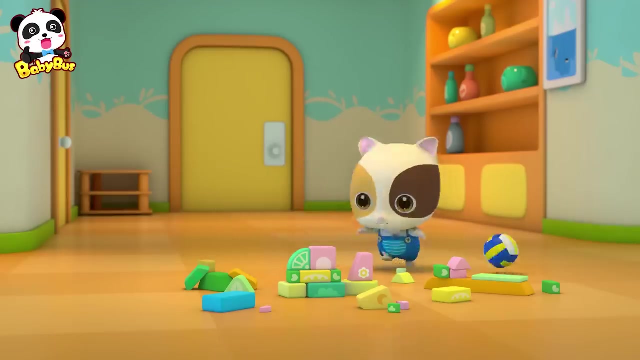 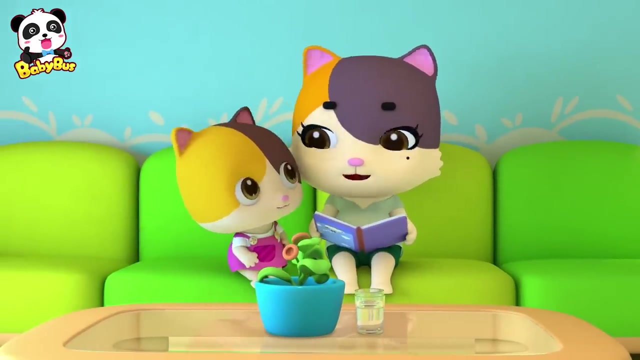 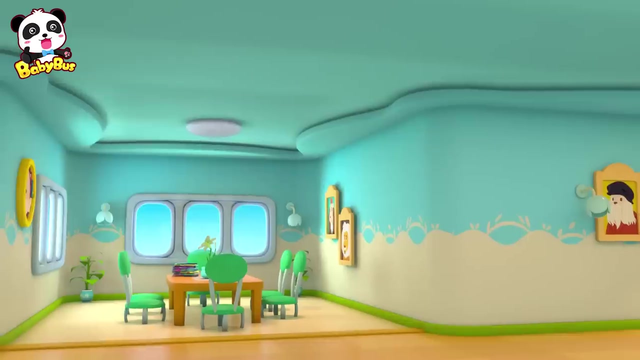 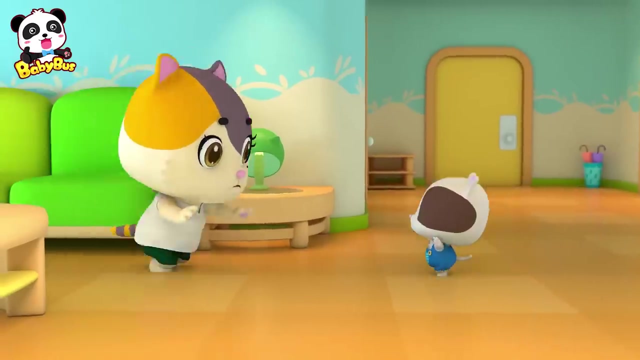 I'm sitting in my safety seat, so I'll be safe too. Yeah, I love my safety seat. Ha ha ha. Mom, what's happening? It's an earthquake. Mimi Timmy, come here. Oh, do you know what to do during an earthquake? 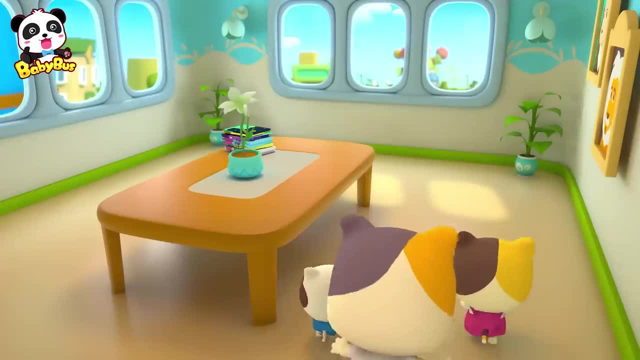 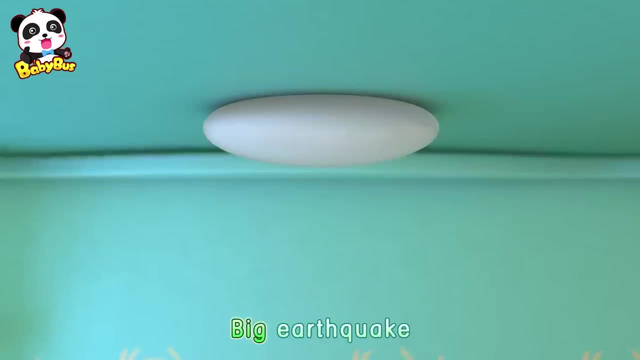 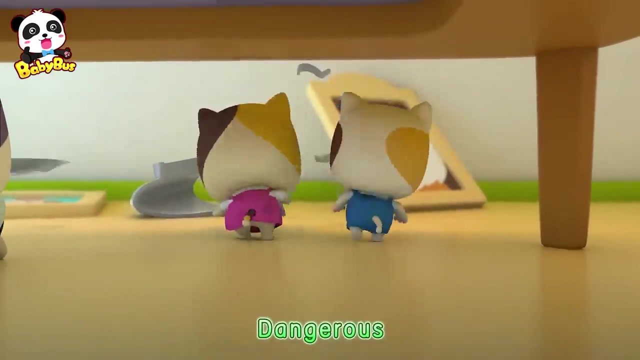 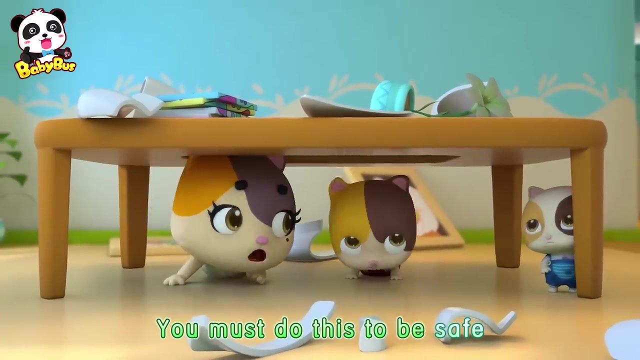 Yes, Big earthquake shaking, shaking. Big earthquake. big earthquake, Dangerous, shaking, shaking, Dangerous, dangerous. Stay calm, please Hide somewhere and crouch down. Hold on tight with your hands. You must do this too. Big earthquake shaking, shaking. Big earthquake, shaking, shaking. 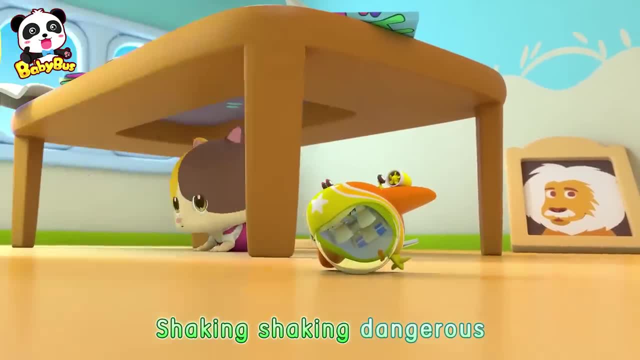 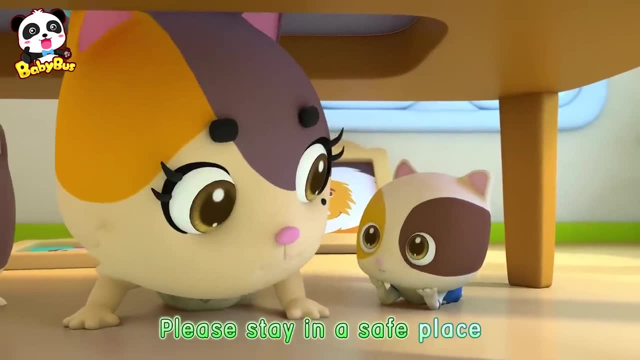 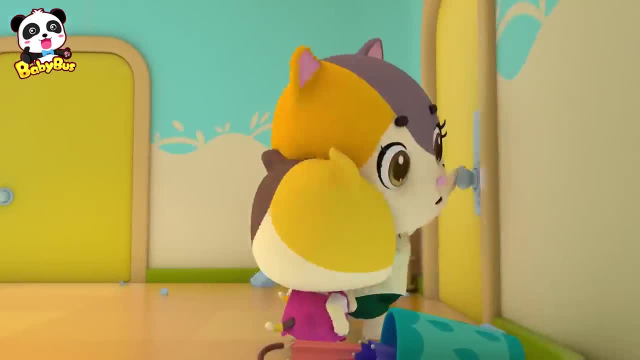 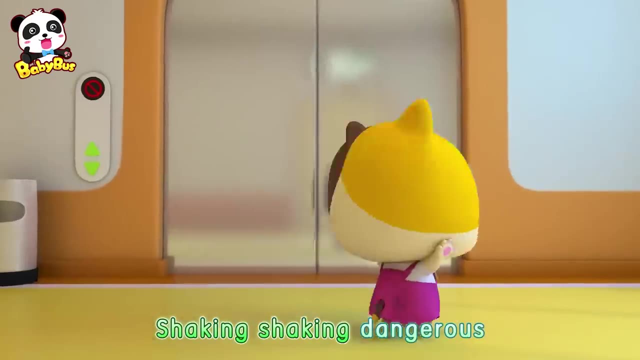 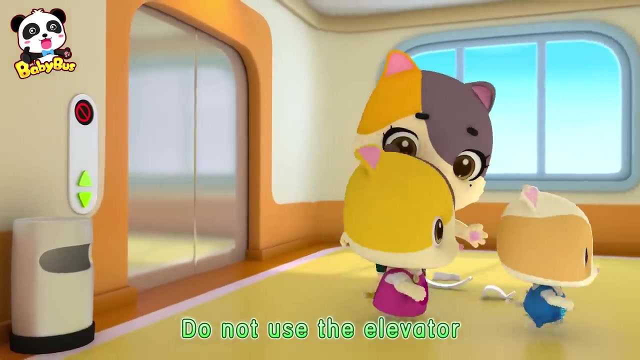 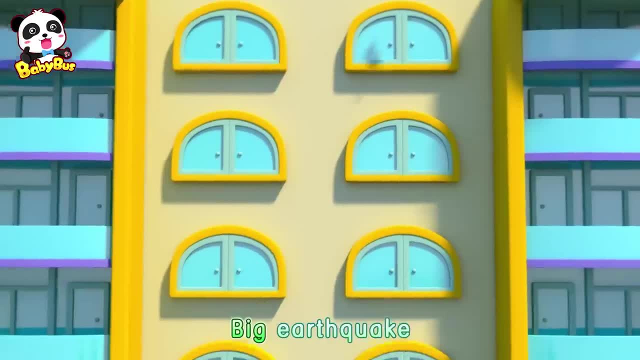 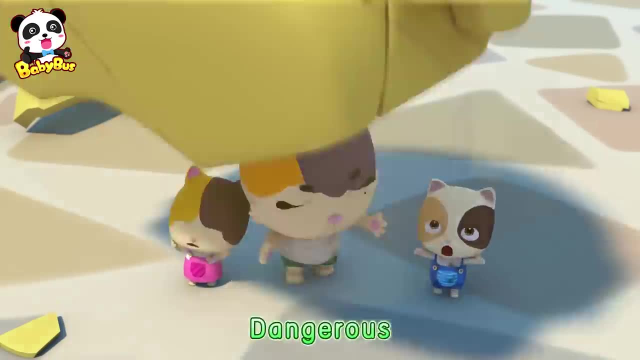 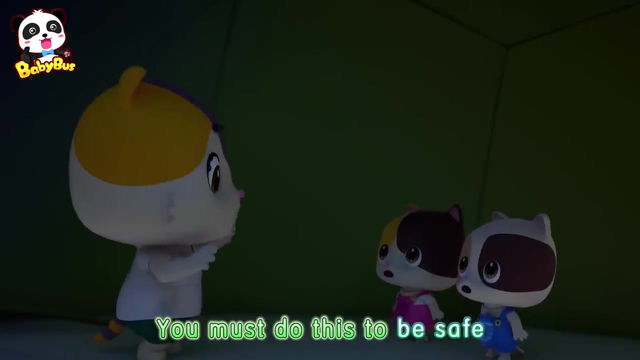 You must do this to be safe, To be safe. Big earthquake, shaking, shaking, Big earthquake, big earthquake, Dangerous, shaking, shaking, Dangerous, dangerous. Stay calm, please. you don't need to cry and shout. Just wait for help to come. You must do this to be safe. 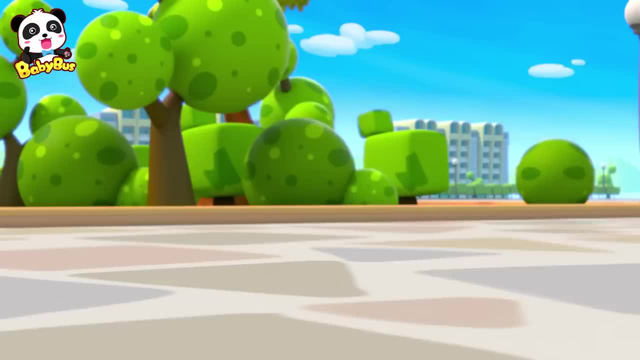 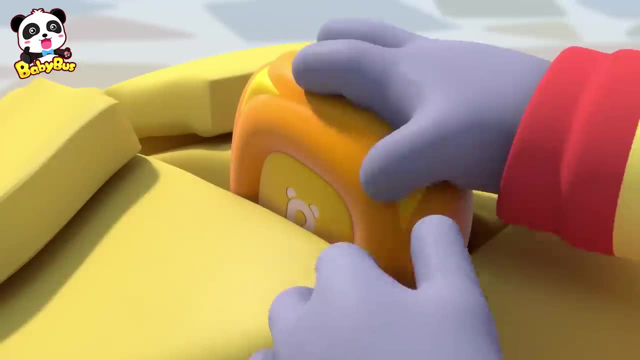 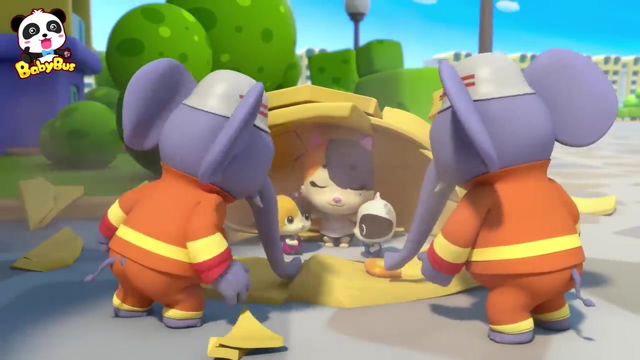 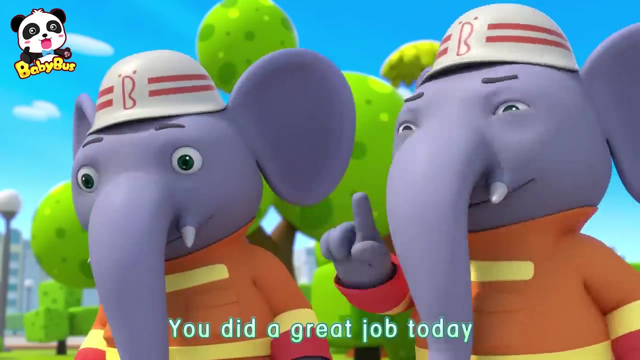 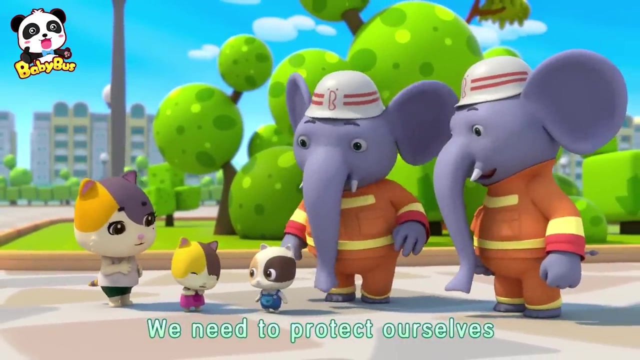 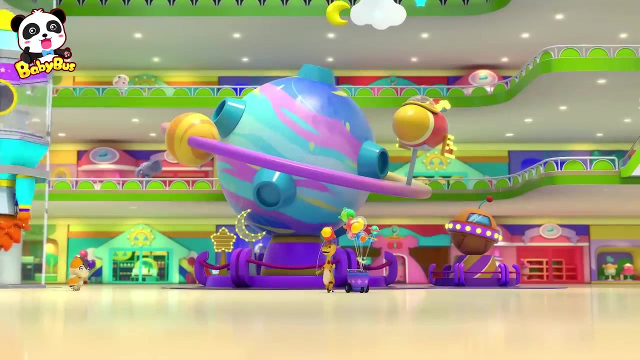 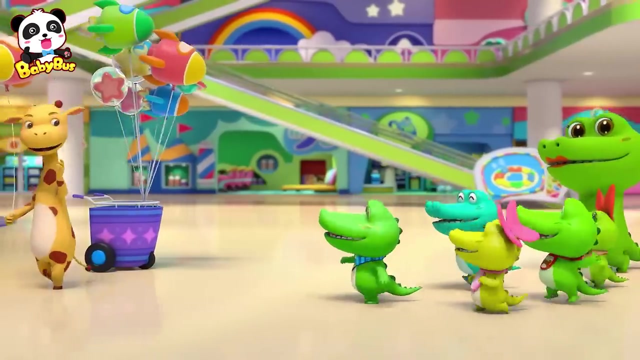 To be safe. Please be safe. Please be safe. Is everyone okay? Thank you, firefighter elephant. You're welcome. You did a great job today. When there's an earthquake, we need to protect ourselves. You're right. Wow, it's wonderful. Wow, mom, we want rocket balloons. 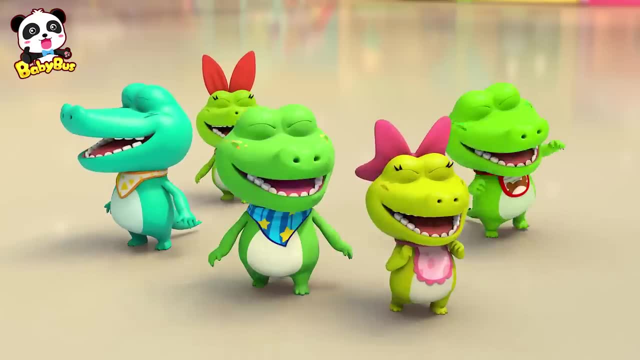 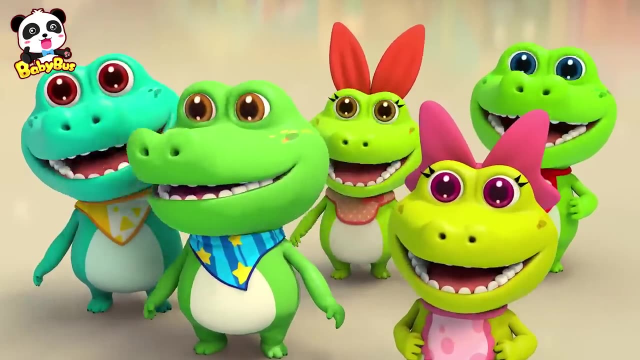 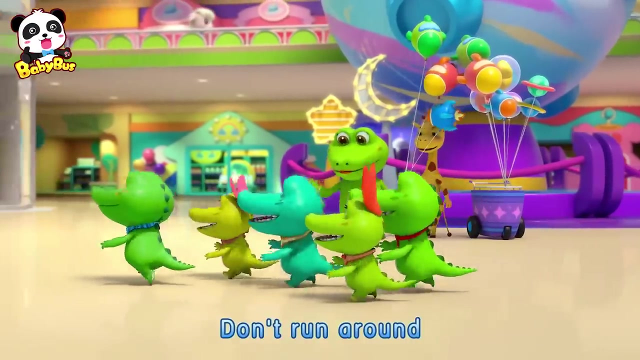 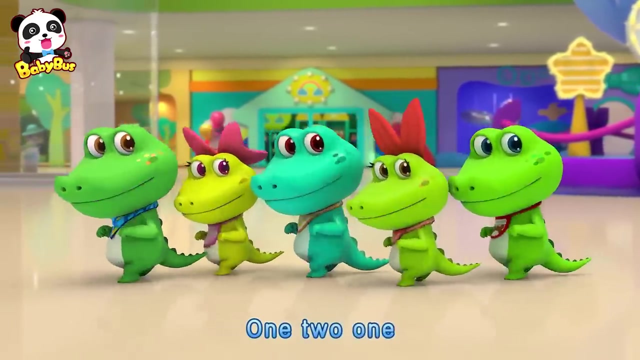 Okay, I like this place. Look over there. Wow, there is a rocket balloon, A bigger rocket over there. Let's get on it, Don't run around. One, two, one, One, two, one, Five little crocodiles. Ha ha, ha, ha, ha ha. 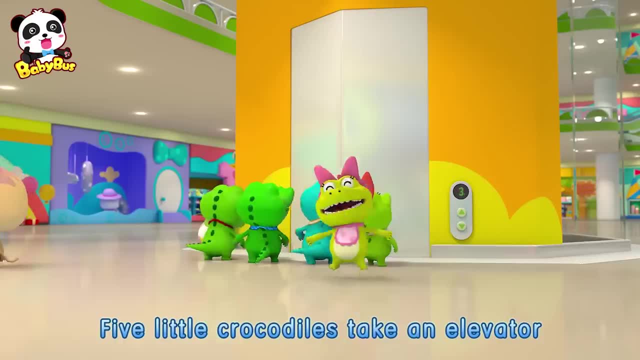 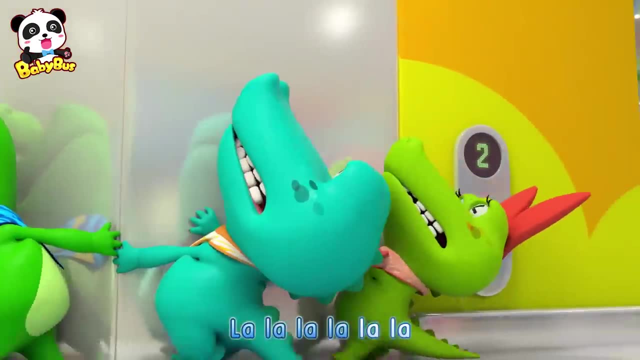 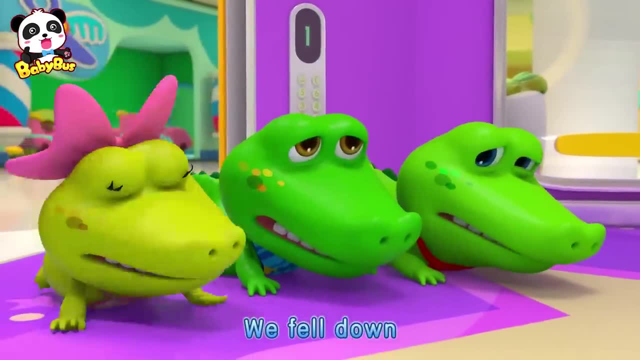 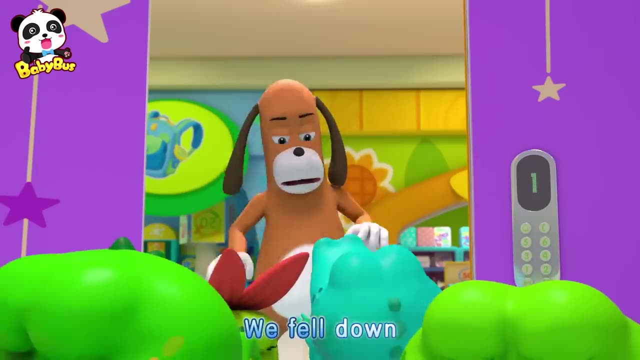 Ooh, ooh, ooh, ooh. we fell down. Ooh, ooh, ooh, ooh, ouch, ouch, ouch, Ooh, ooh, ooh, ooh. we fell down. Ooh, ooh, ooh, ooh, ouch, ouch, ouch. 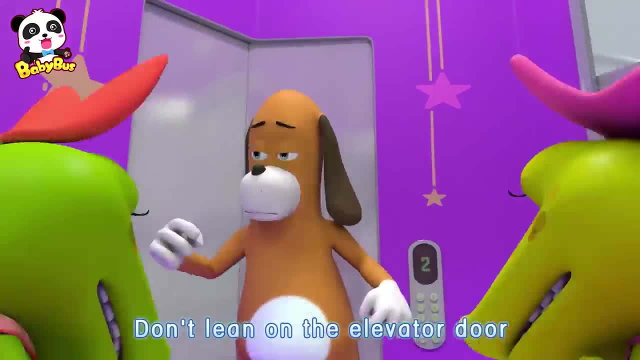 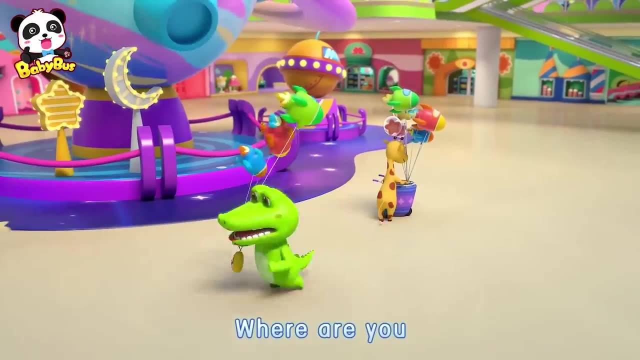 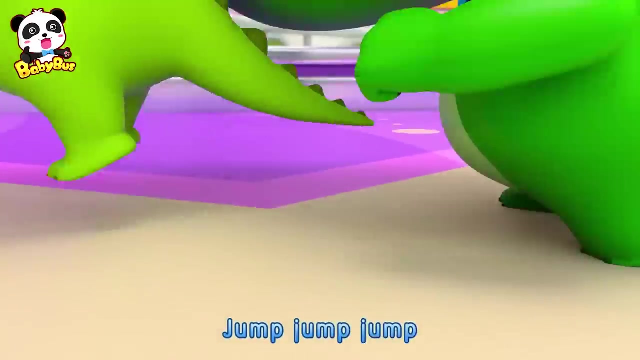 Don't lean on the elevator door. It's dangerous, You could get hurt. Where are my babies, Kids, where are you? It's Mommy, Jump, jump, jump, Jump, jump jump. Let's push the button. 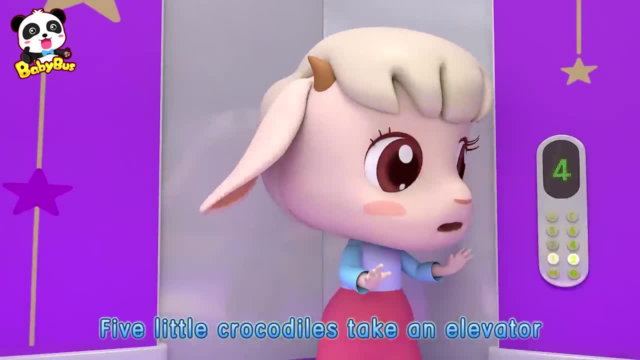 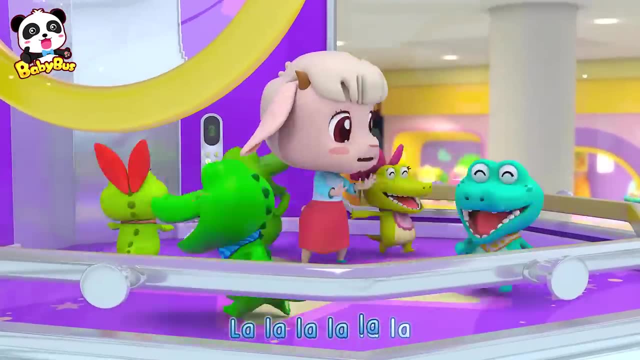 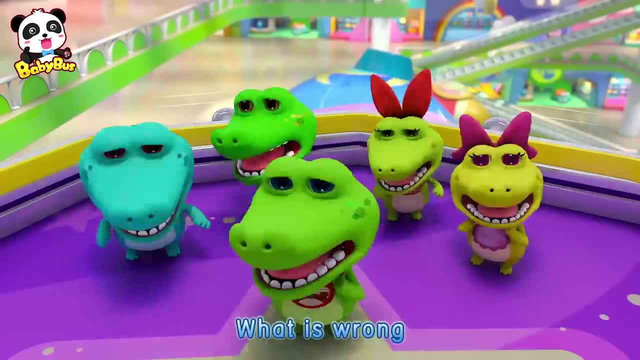 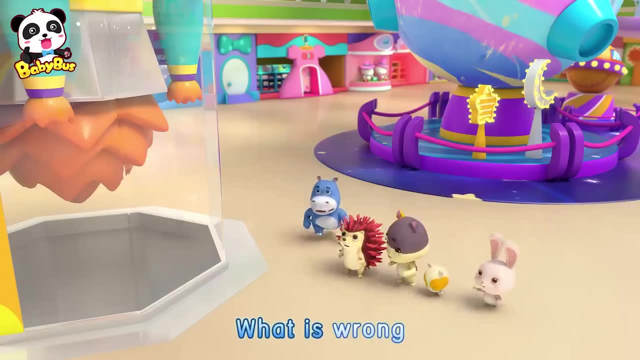 Ooh, ooh, ooh, ooh, what is wrong? Ooh, ooh, ooh, ooh, we are scared. Ooh, ooh, ooh, ooh, what is wrong? Ooh, ooh, ooh, ooh, we are scared. 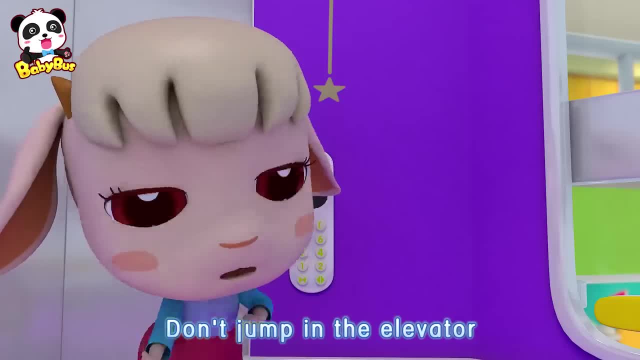 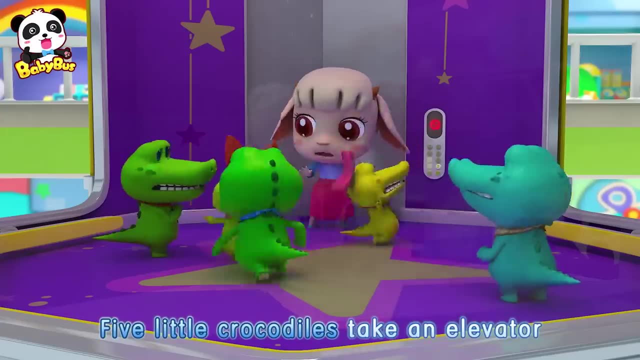 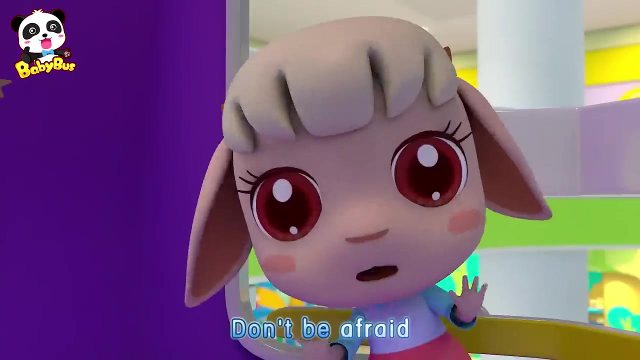 No, no, don't jump in the elevator and don't push too many buttons either. Ah, I'm scared. I want my mommy. Five little crocodiles take an elevator. It is broken. What should we do? Don't be afraid. Please stay calm. Push the emergency button and 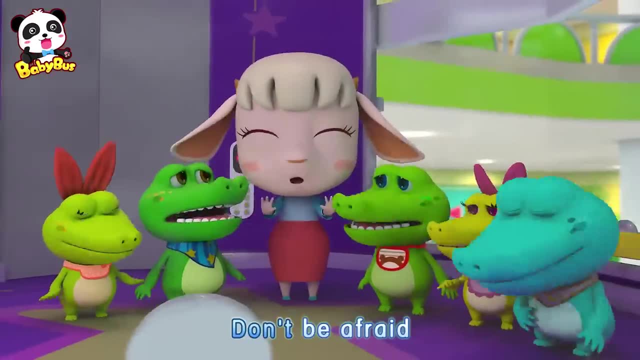 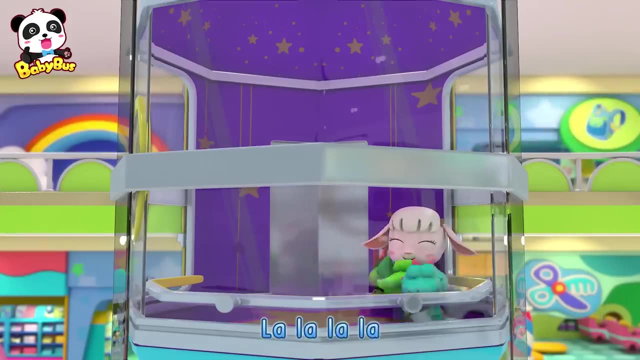 Wait for help. La la la la. don't be afraid. La la la la. please stay calm. La la la la, we'll be all right. La la la la help arrive. 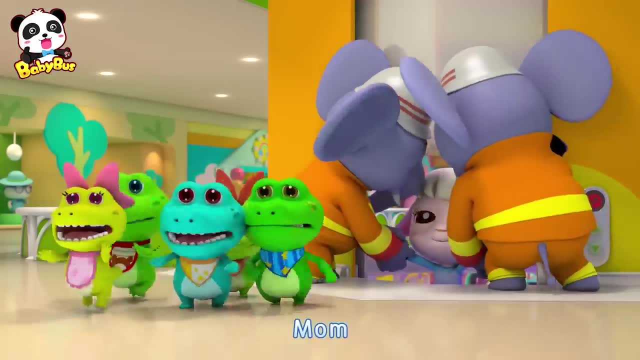 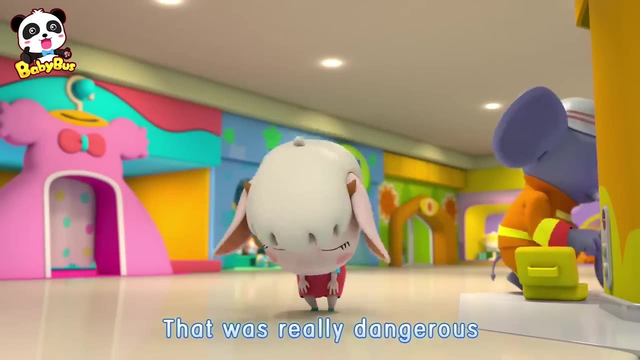 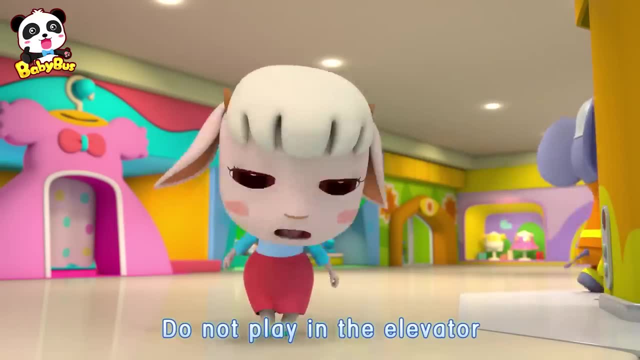 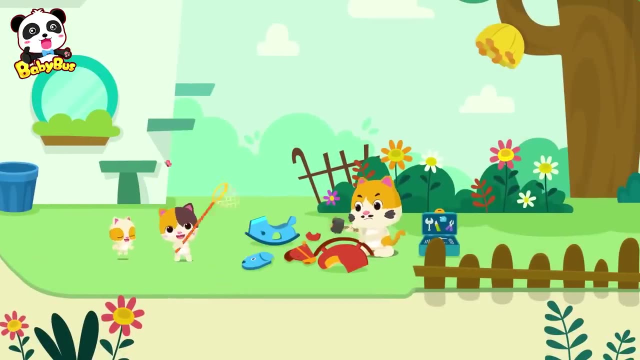 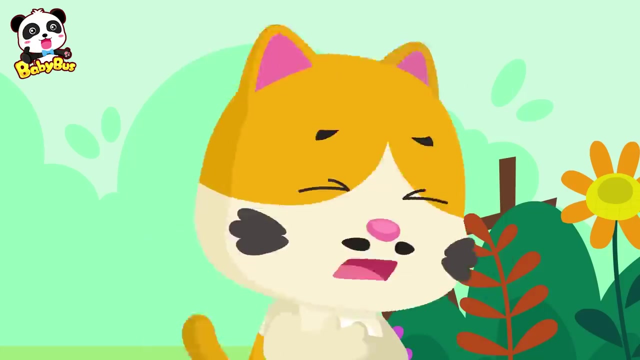 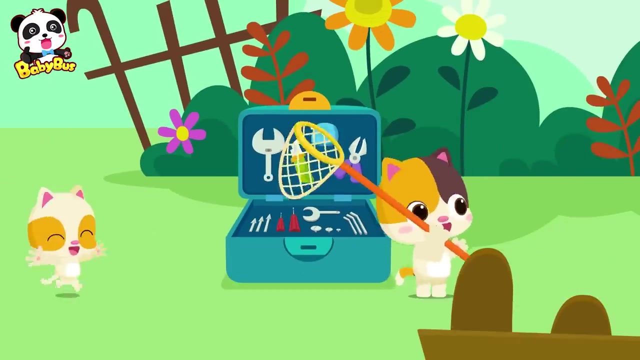 Phew, Phew. It's really dangerous. Kids do not play in the elevator like the little crocodiles. Ow, That hurts. I need a bandage. Huh, Huh, Wow, Timmy, look at these toys. 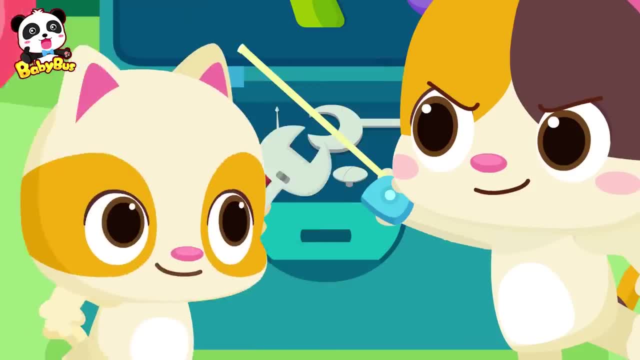 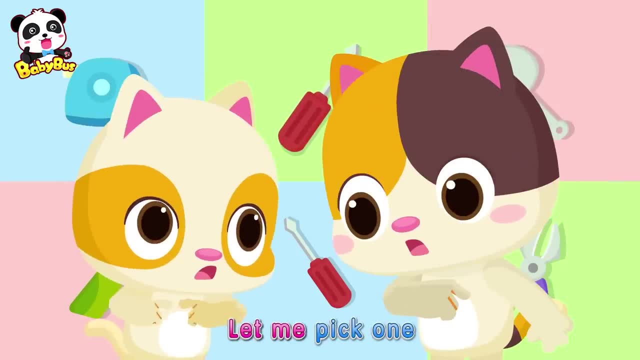 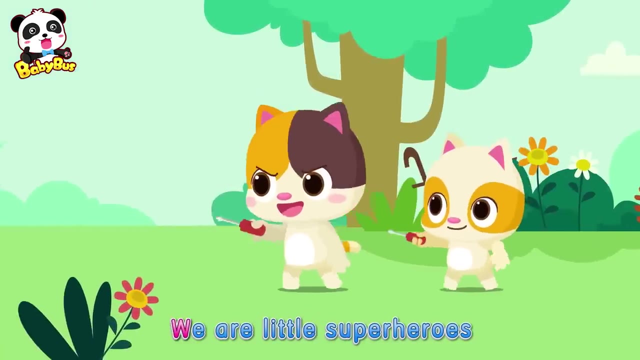 Let's play with them. Okay, Wonderful toy, Let's take a look. Let me pick one. I like this one. I like this one. Lululala, we are little superheroes. Lululala, let's fight the big monster. 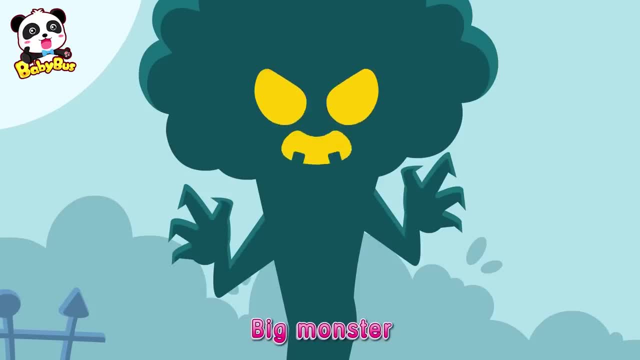 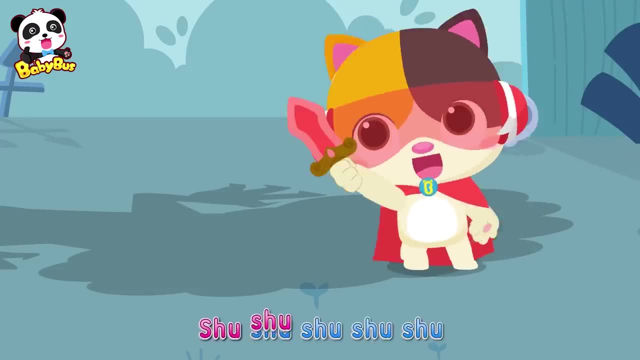 Big monster, We're not afraid. Hoo-hoo-hoo, Ha-ha. See how brave I am. Shoo-shoo-shoo-shoo-shoo. I hurt my leg, Ow-ow-ow, Ow-ow-ow. 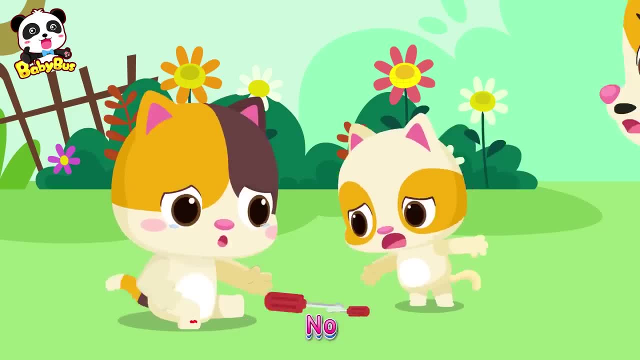 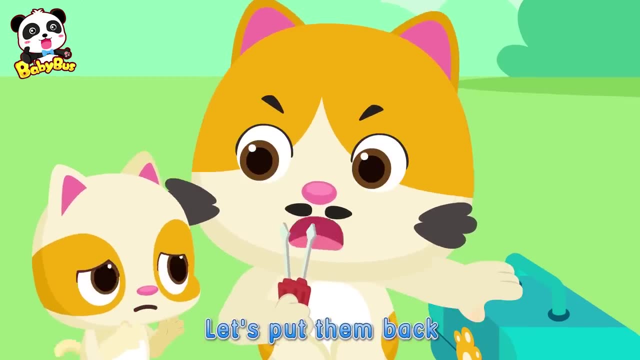 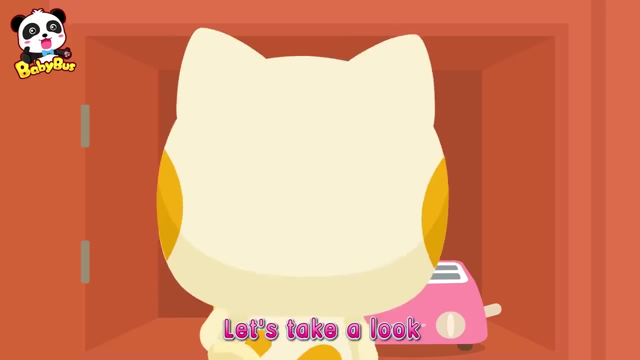 It is so pointy. It's not a toy. no, These are tools. They're dangerous. Don't play with them. Let's put them back. Wonderful toys- Let's take a look. Let me pick one. I like this one. 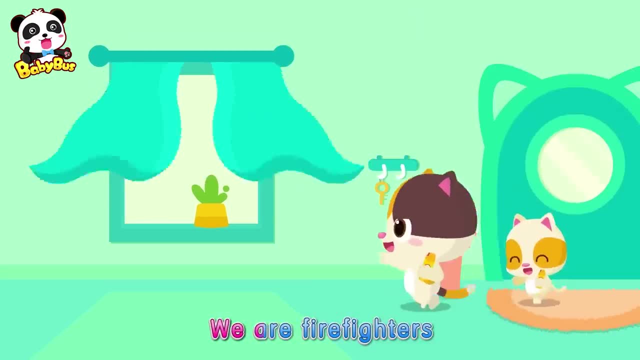 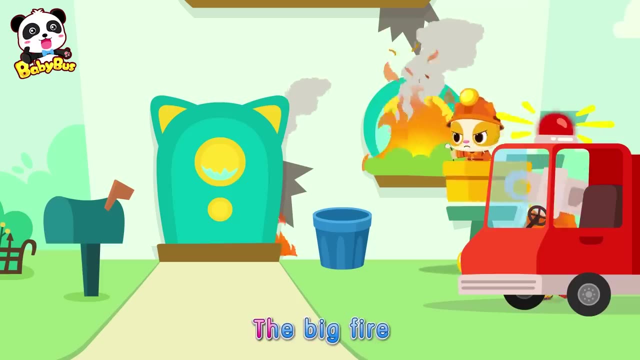 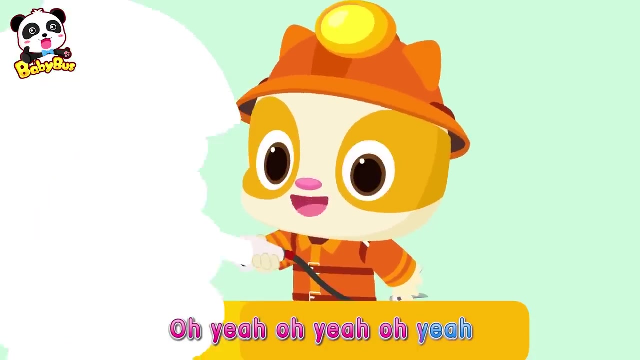 It's not pointy at all. Lululala, we are fire fighters. Lululala, let us put out the fire, The big fire. To the fire up there. Oh yeah, oh yeah, Oh yeah, to the fire down there. 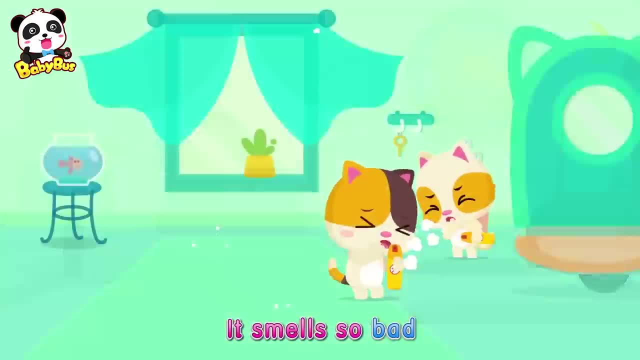 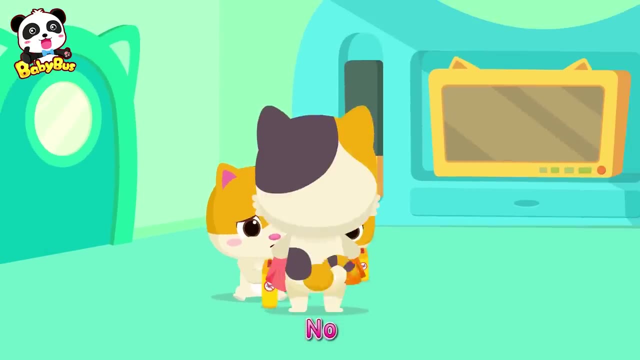 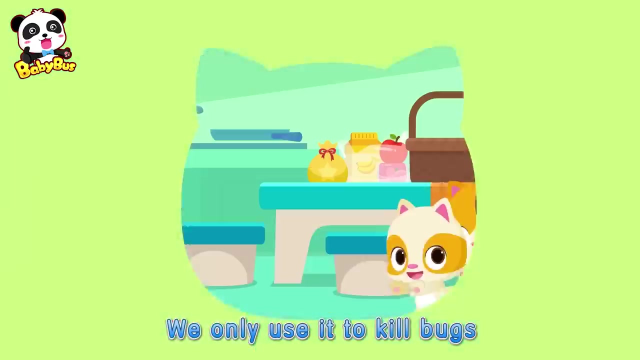 Yeah, yeah, yeah, yeah, yeah, yeah. It smells so bad. Smelly, smelly, ew, ew. The smell is really bad. It's not a toy. no, This is bug killer. It's dangerous. don't play with it. We only use it to kill bugs. 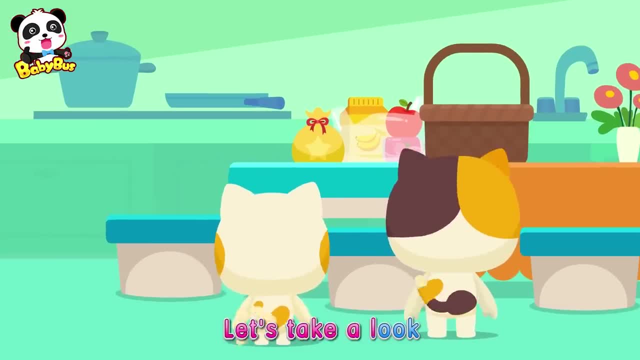 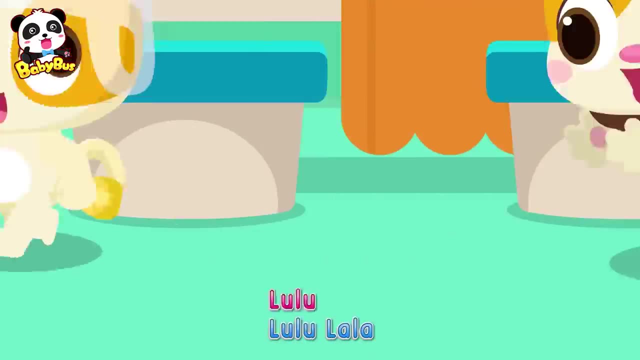 Ba-da-ba-ba-ba- wonderful toys. Let's take a look, Ba-da-ba-ba-ba, let me pick one. I like this one. It doesn't smell bad. Lululala, let's play Cops and robbers. 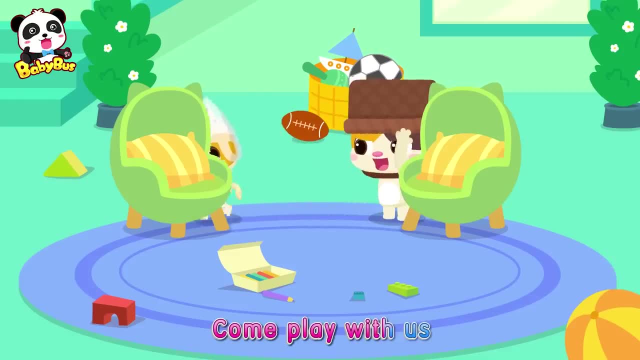 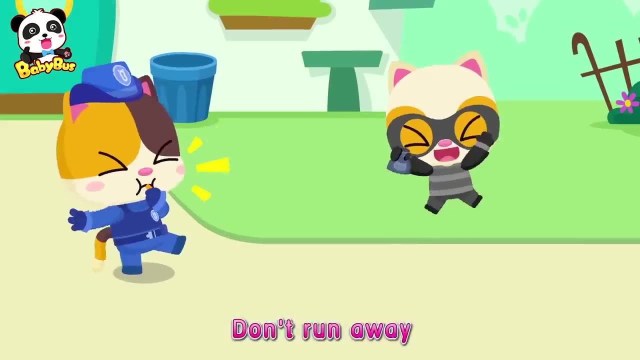 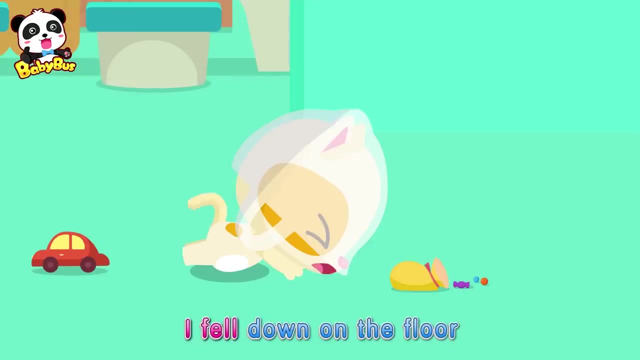 Lululala, everyone, Come play with us. I got you. Stop, don't run away. Hey, hey, hey-ho, You can't catch me. Hey-ho, hey-ho, hey-hey. I fell down on the floor. Oh-oh-oh, oh-oh-oh. 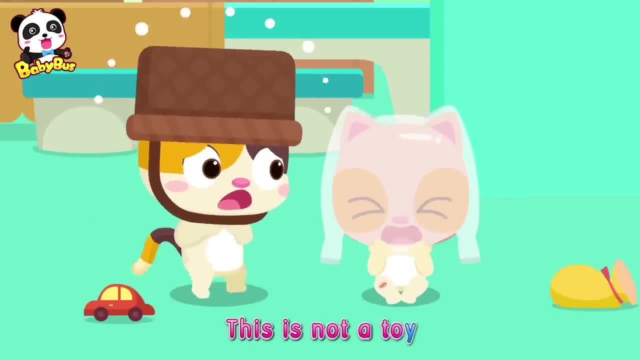 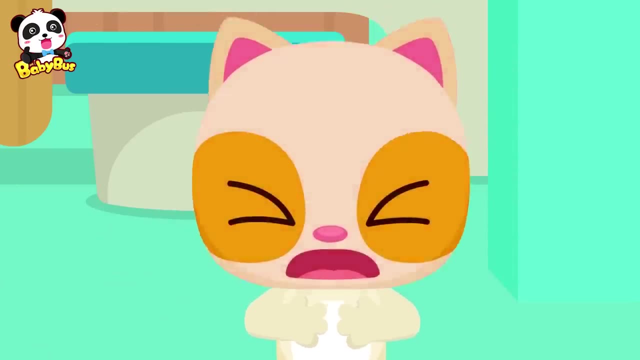 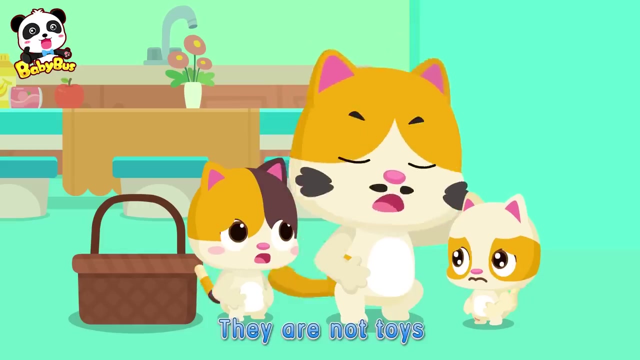 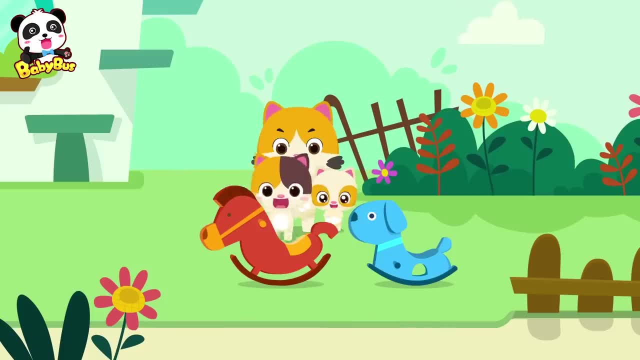 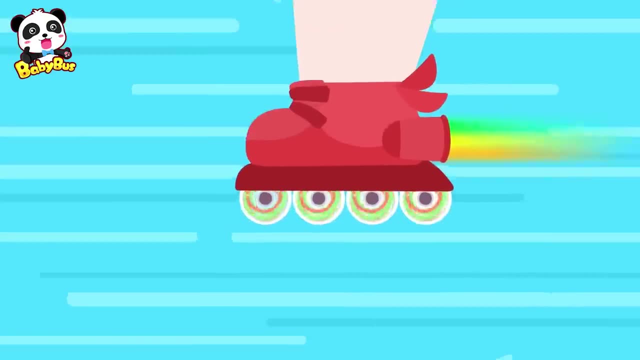 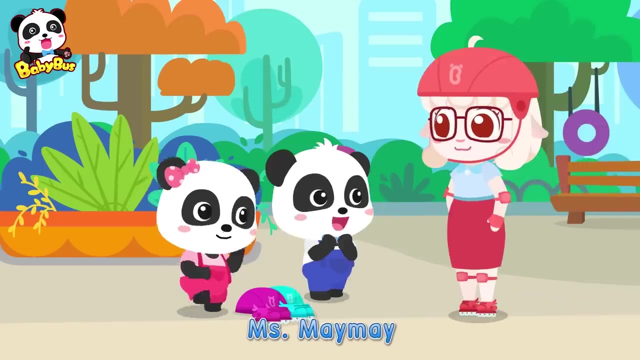 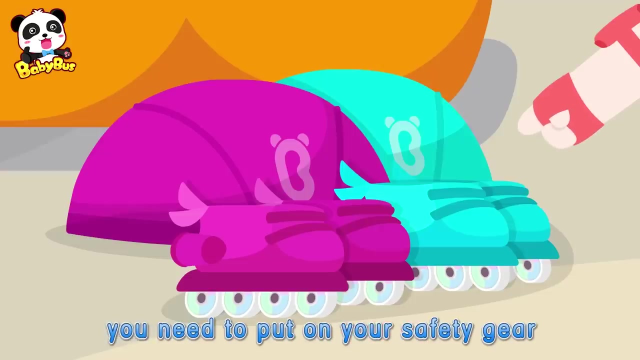 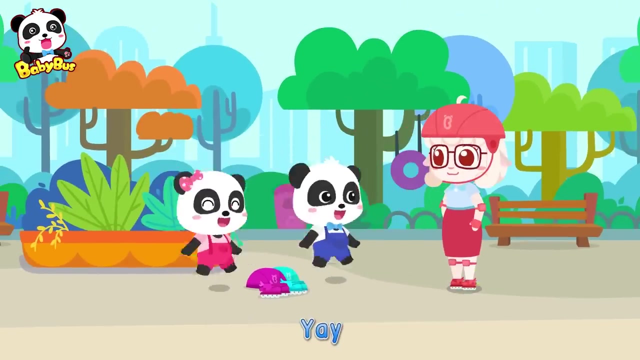 Your toys are right here. Wow, Wow, wow. Ms Mei Mei, can you teach us how to skate? Of course, But first you need to put on your safety gear. Okay, Let's skate together. Yay, We like skating, it's so fun. 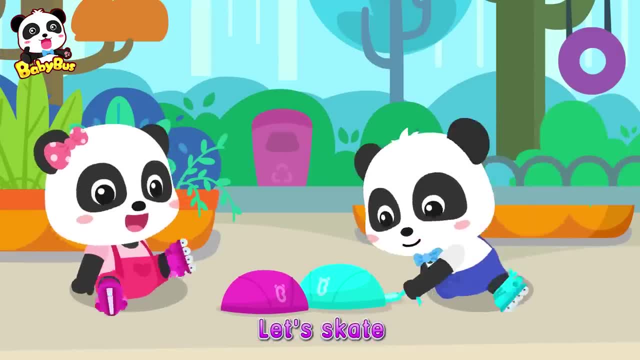 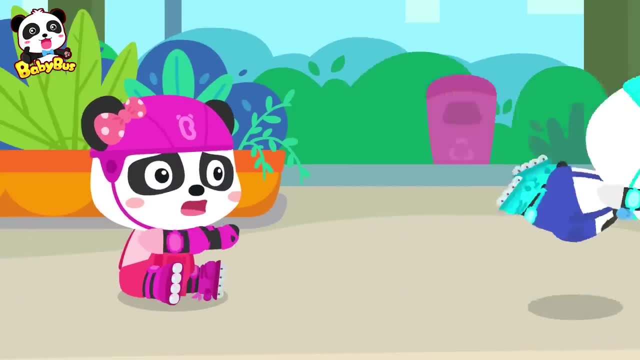 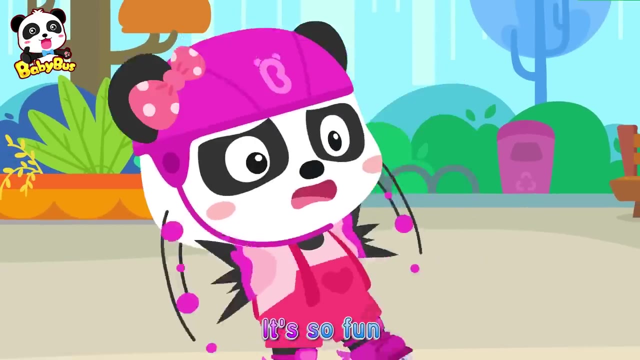 Let's skate, let's skate. Put on your knee pads and wrist pads. Put on your helmet too. Ouch, Don't worry, you have safety gear. Okay, We like skating, it's so fun. Let's skate, let's skate. 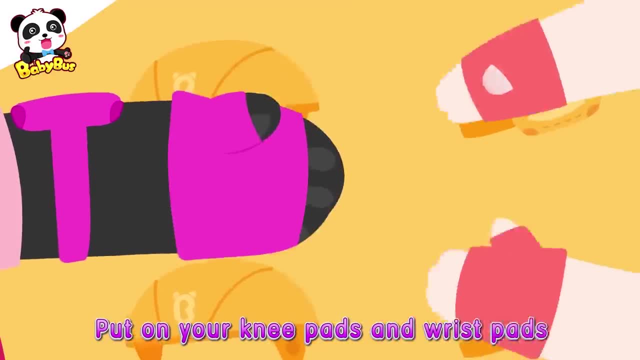 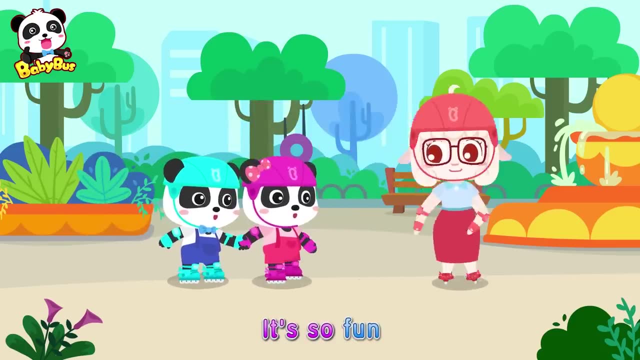 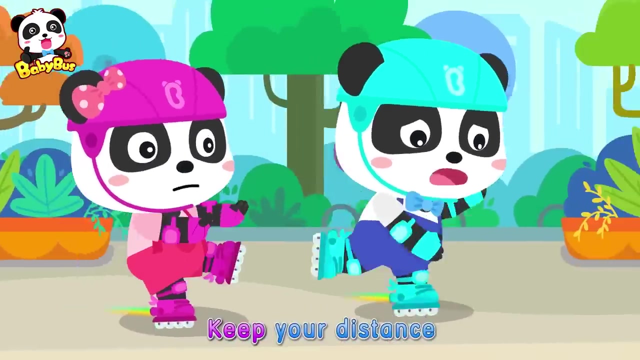 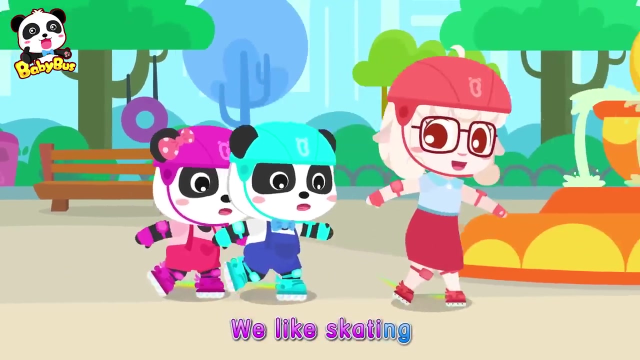 Put on your knee pads and wrist pads. Put on your helmet too. We like skating, it's so fun. Let's skate. let's skate. Spread your arms, keep your distance. Come on, here we go. We like skating, it's so fun. 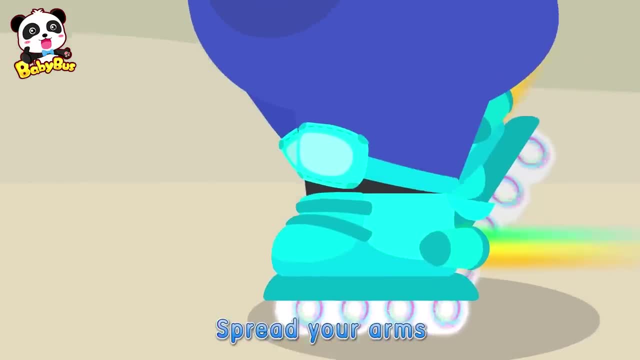 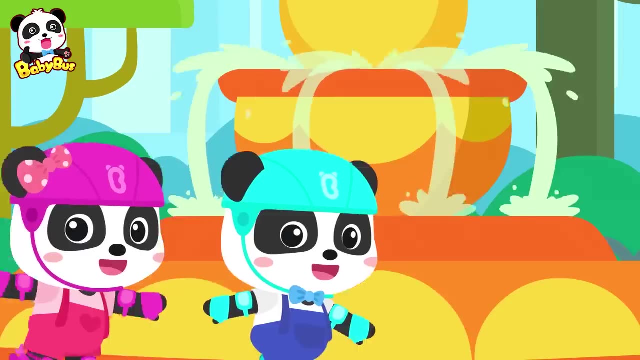 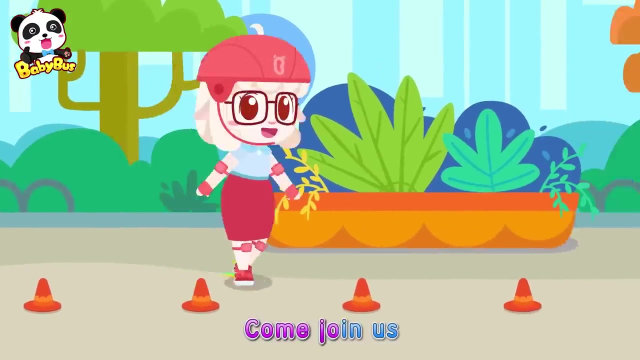 Let's skate, let's skate. Spread your arms, keep your distance. Come on, here we go. We can skate now. Let's go, Let's go, Come join us. it's so fun. Let's skate, let's skate. 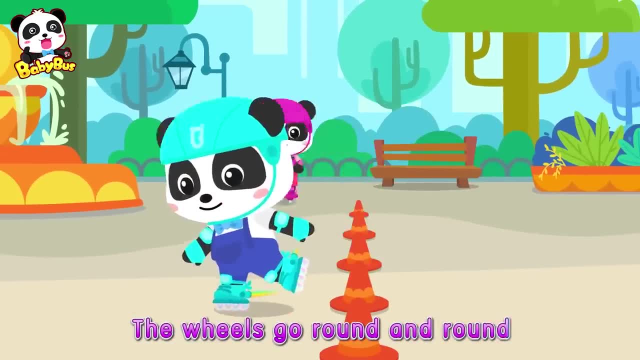 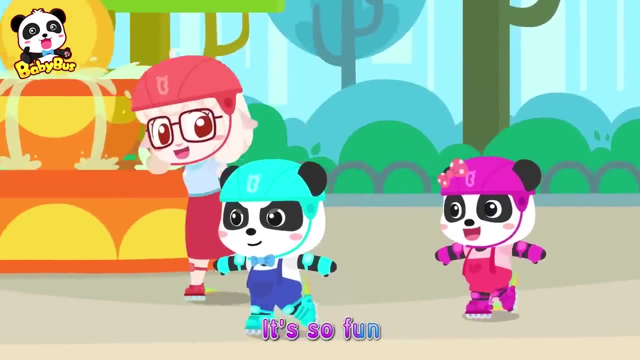 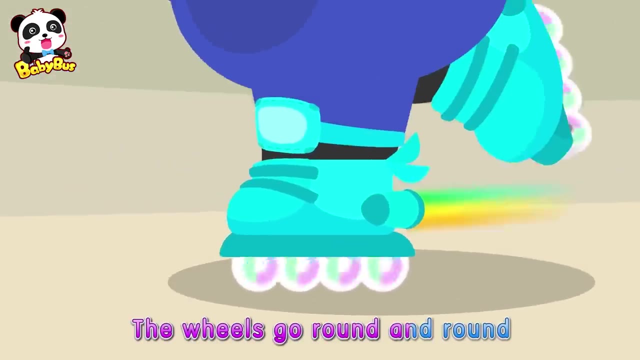 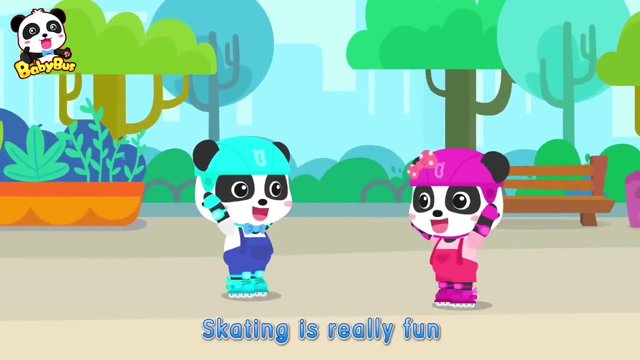 The wheels go round and round, Shiny shiny. Come join us, it's so fun. Let's skate, let's skate. The wheels go round and round, Shiny shiny, Shiny shiny. Skating is really fun, Yeah. 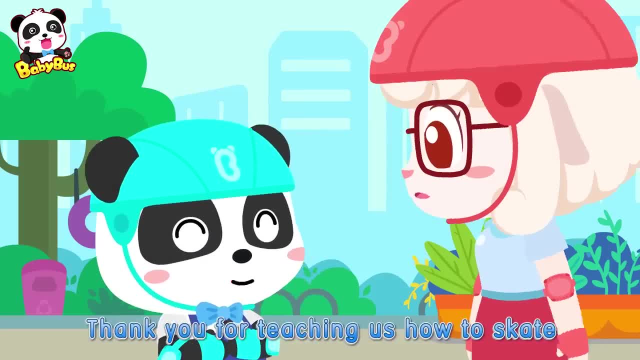 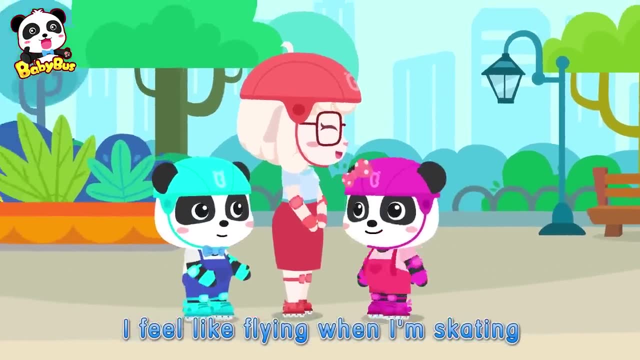 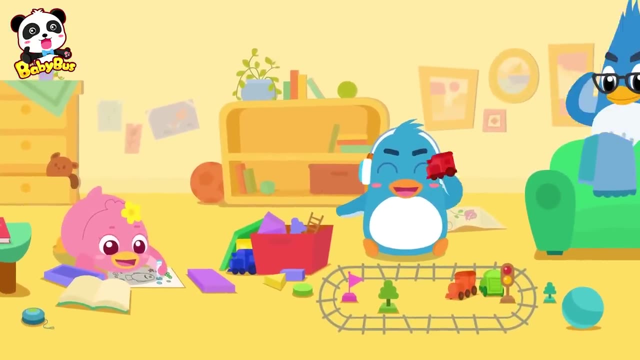 Miss Mimei, thank you for teaching us how to skate. Yeah, I feel like flying when I'm skating. You're welcome. Let's do it again next time. Okay, Choo-choo, Choo-choo. Don't forget to clean your room. 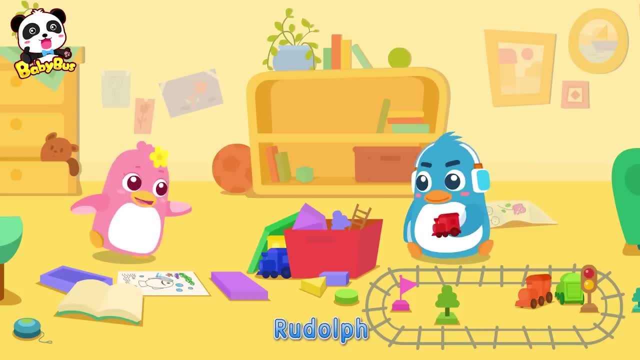 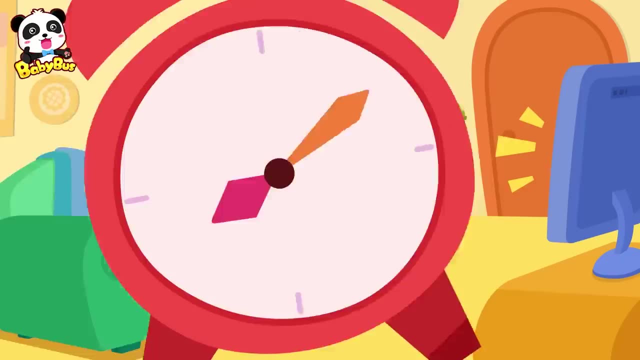 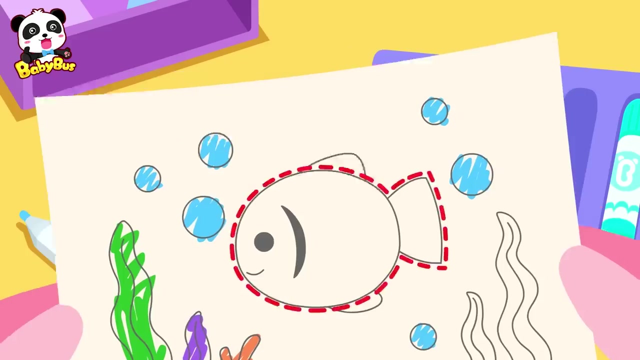 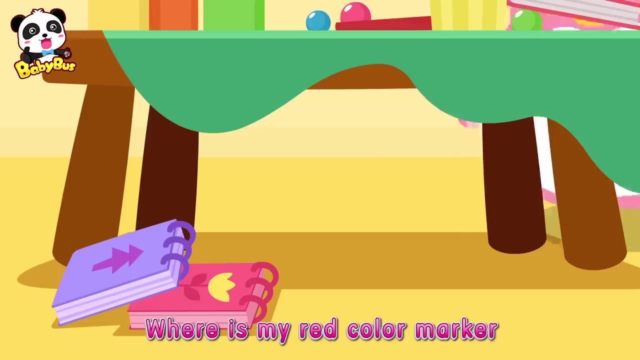 Clean your room. Okay, Then off the cartoonist Artie. Yeah, let's go. That was really fun, Let's go play again. Color marker, color marker. Where is my red color marker? I can't find you. where are you? 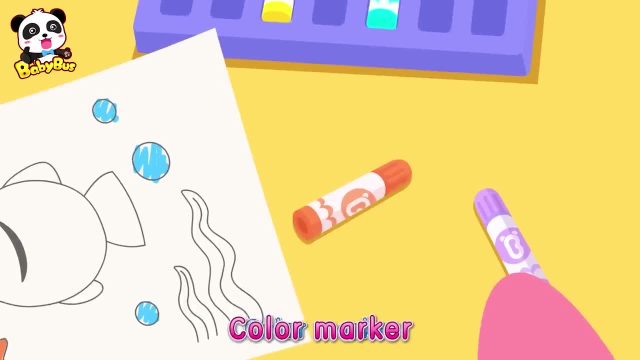 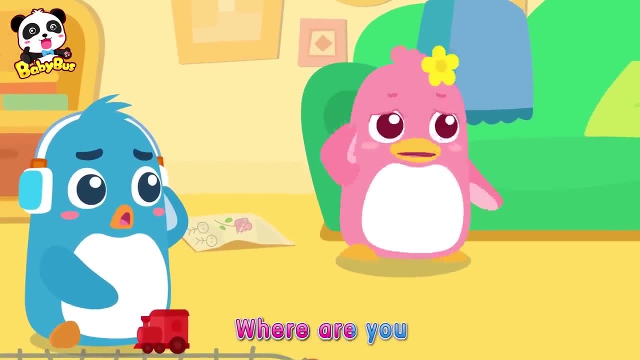 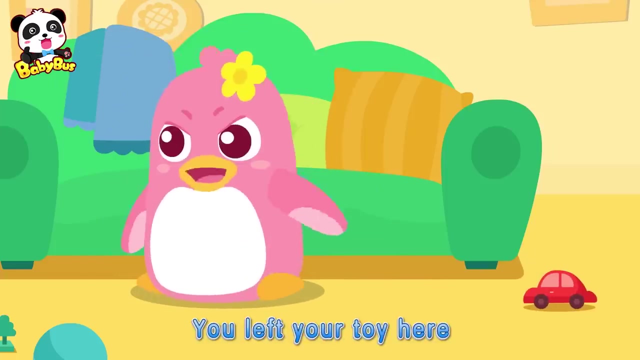 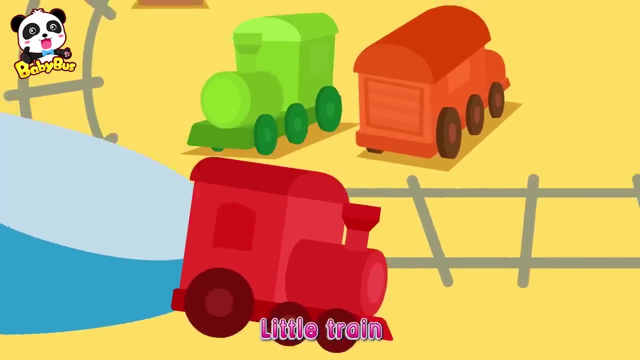 I need you right now. Color marker, color marker. Where is my green color marker? I can't find you. where are you? I won't drop you anymore. Rudolph, you left your toy here, Sorry. Little train, little train. 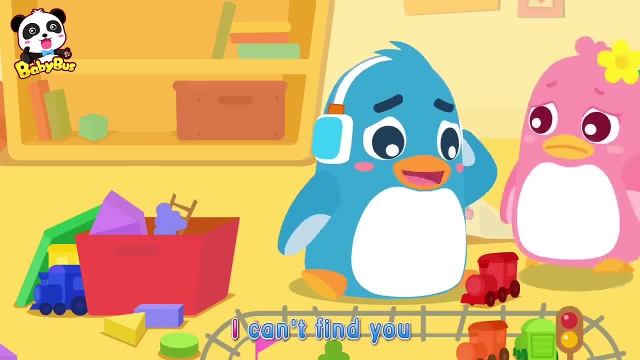 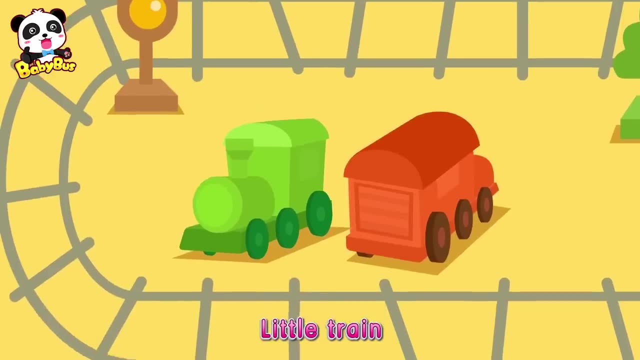 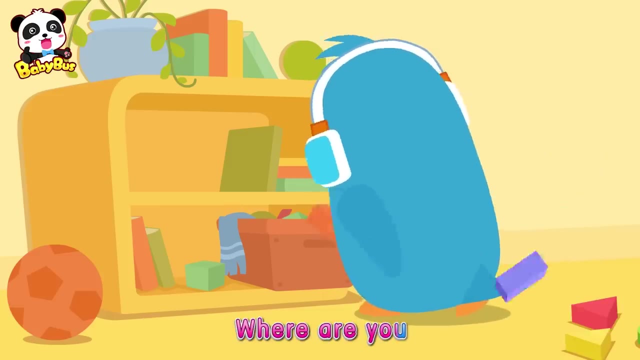 Where is my blue little train? I can't find you. where are you? I need you right now. Little train, little train. Where is my yellow little train? I can't find you. where are you? I won't drop you anymore. 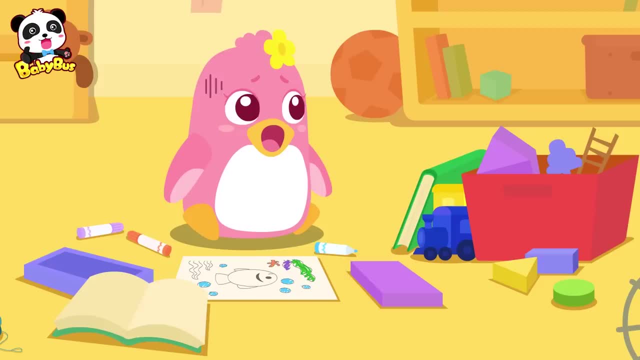 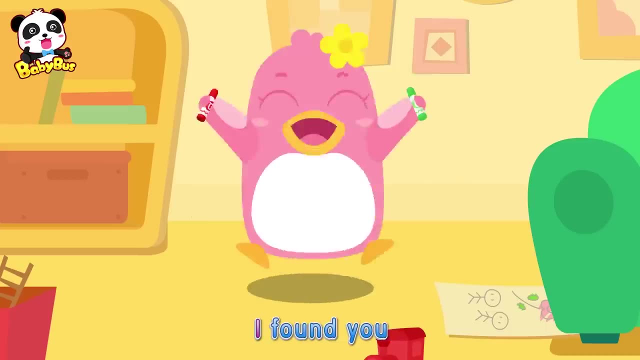 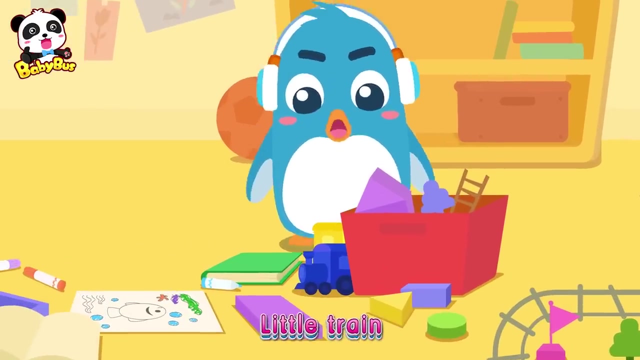 Rudolph, you left your toy here, Sorry. Color marker. color marker: Red and green color marker. I need you right now. Where are you? Where are you? I found you? yes, I found you. Both of you are right here. Little train, little train. Blue and yellow little train.